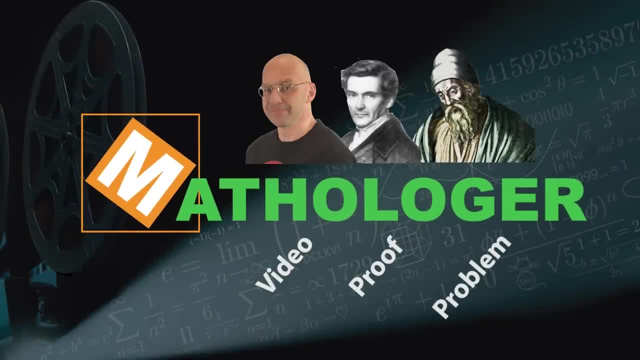 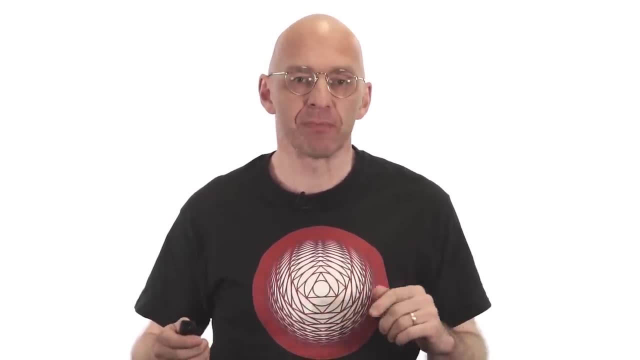 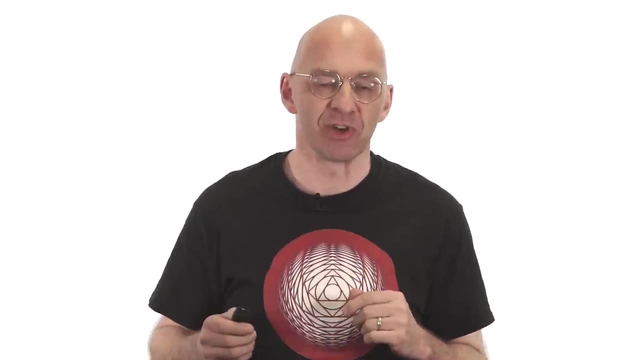 Welcome to another Mathologer video. Today's video is one I've been dreaming about making for a long, long time. Today, I'd like to dazzle you with the solutions of some of the most famous problems in the history of mathematics. These problems had remained unsolved for more than 2,000 years after. 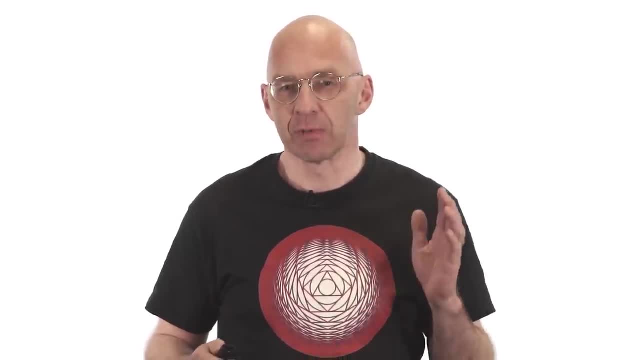 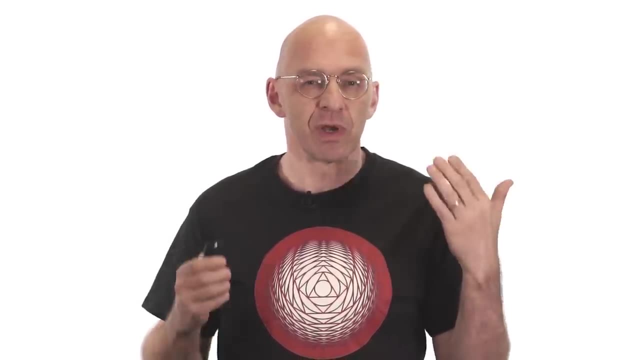 they were first puzzled over in ancient Greece. The problems arose very naturally as part of the Greeks' mathematicians' quest to determine the possible geometric constructions. when all we're permitted is to draw lines and circles, That is what is possible using just the most basic. 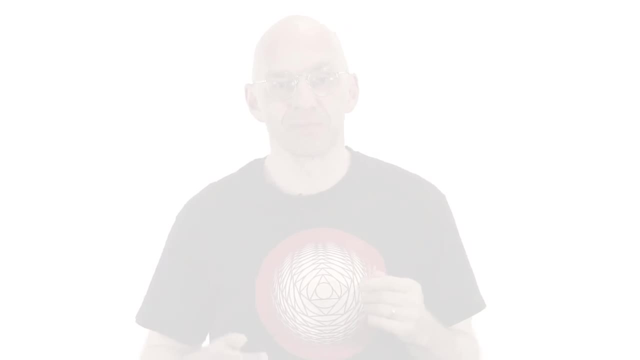 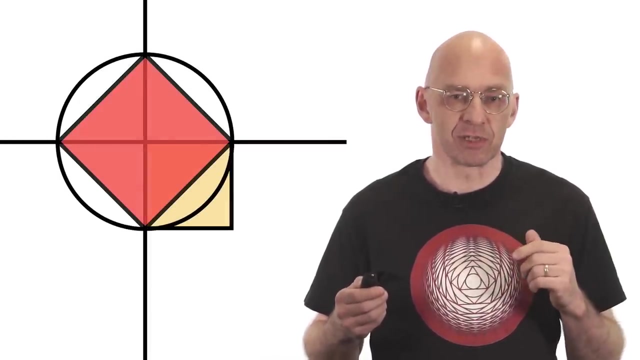 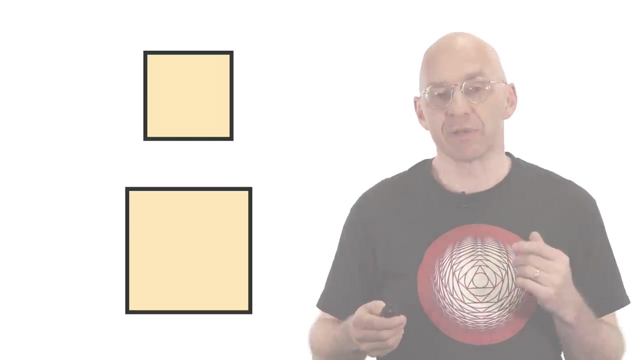 mathematical tools, the ruler and the compass, For example. given a square, we could construct a new square of twice the area just using our basic tools. However, unlike doubling a square like this, doubling a cube turned out to be anything but easy. 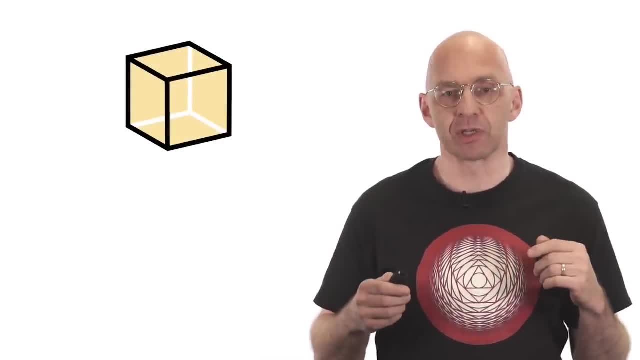 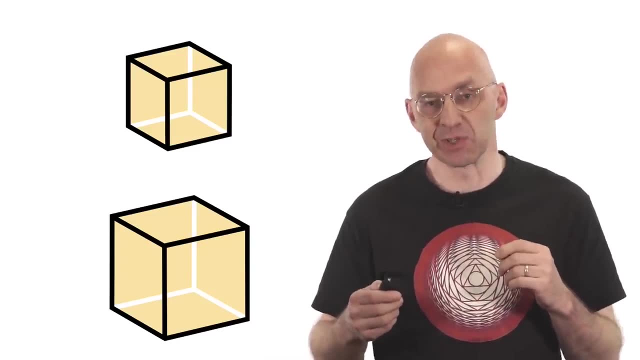 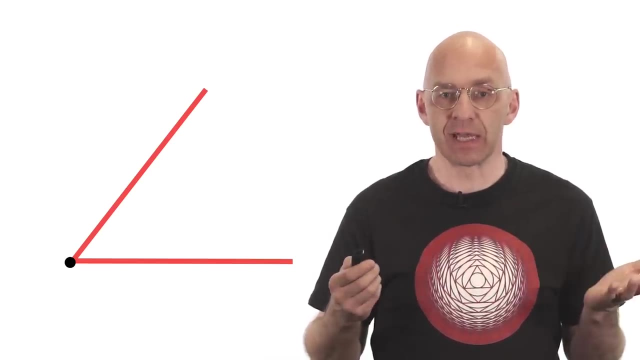 Nobody was able to figure out whether, given a cube, we could construct a cube of double the volume by just using ruler and compass. This is the first of those ancient problems I'll be tackling today. Similarly, if you are given two lines making some angle, then halving that angle with ruler. 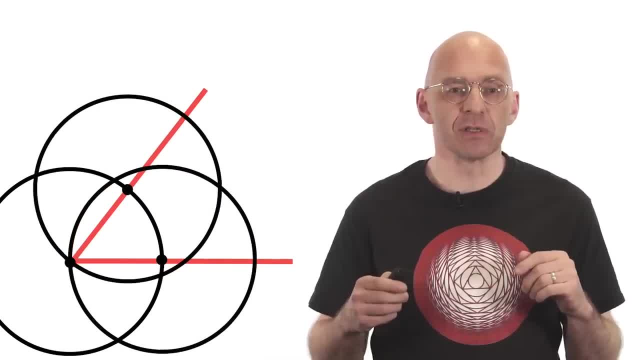 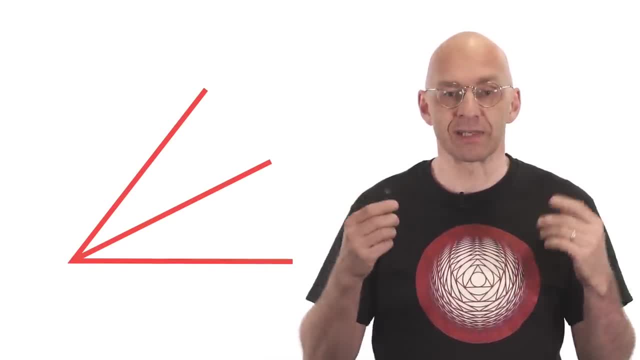 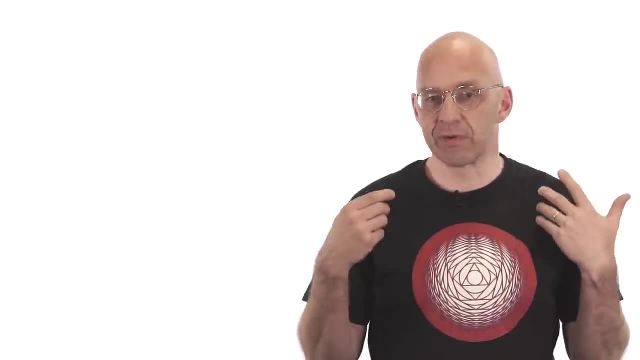 and compass is easy There. just draw a couple of circles There and there is the bisector. But nobody could come up with a ruler and compass construction that would trisect an arbitrary circle. That's problem number two. Next, using ruler and compass to construct equilateral triangles. 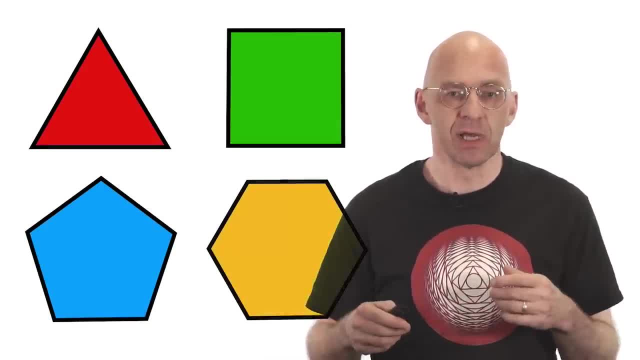 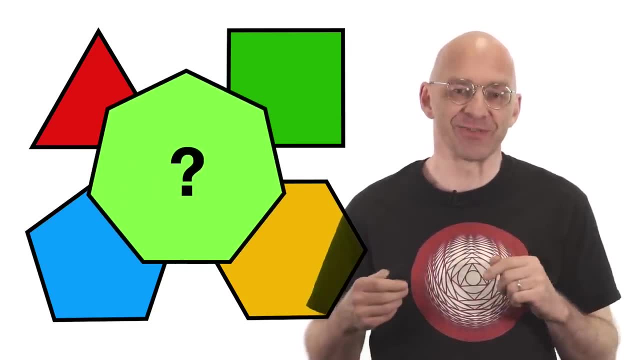 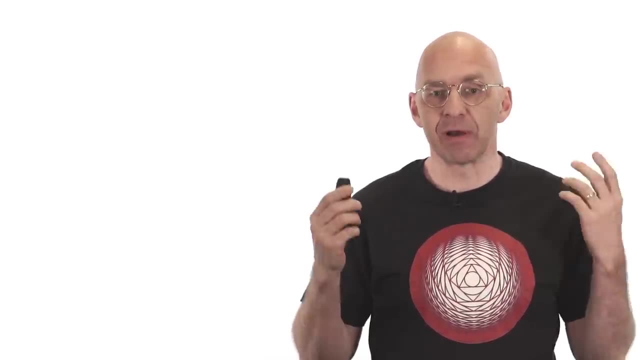 squares. regular pentagons and regular hexagons is not a problem at all, But what about regular heptagons? Nobody had a clue for thousands of years. That's problem number three. Finally, most famously, and what turned out to be by far the hardest, 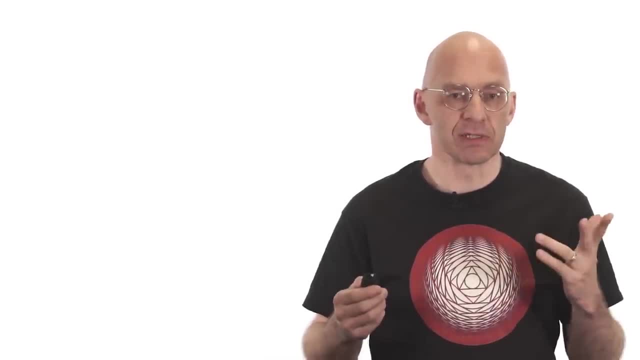 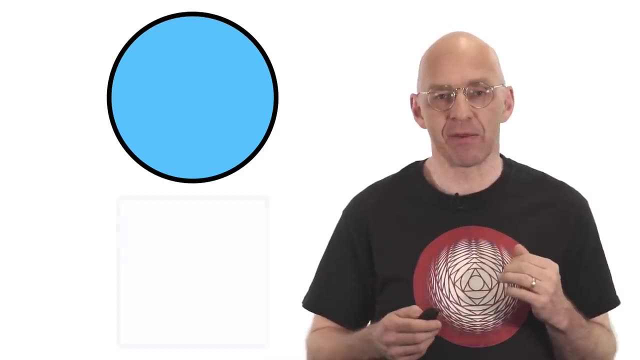 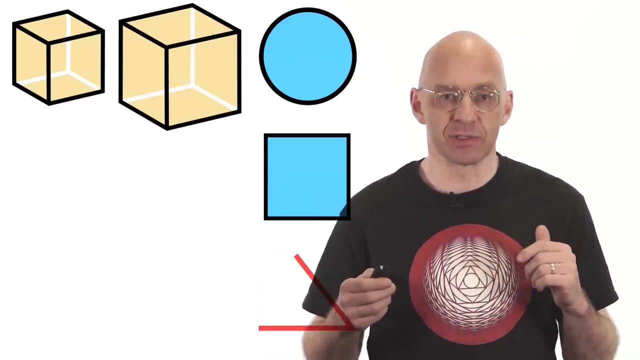 is it possible to square a circle That is Given a circle? is it possible to use ruler and compass to construct a square of exactly the same area? Well, as I said, it took over 2,000 years to finally answer these questions. And what's the answer? The answer is: stop trying, you're. 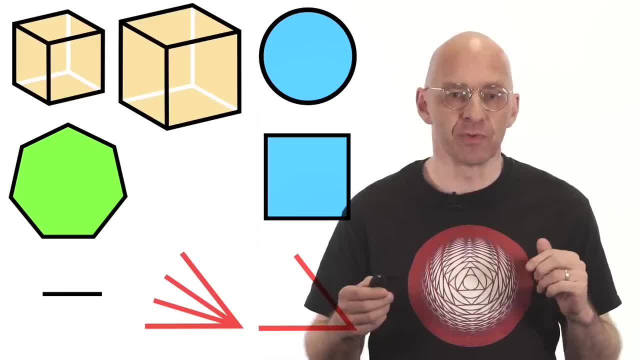 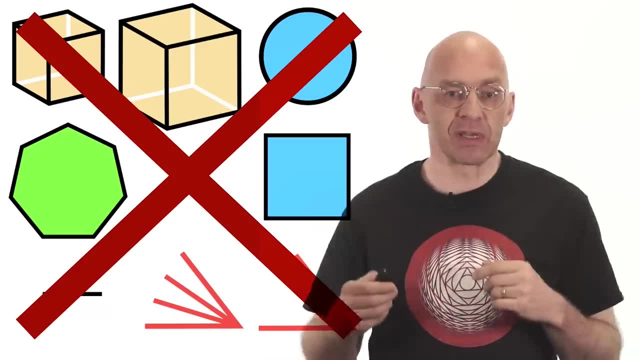 wasting your time. In the 19th century it was proved that it's impossible to use ruler and compass to double a cube or to trisect an arbitrary angle, or to construct a regular heptagon or to square a circle. But who gets to see? 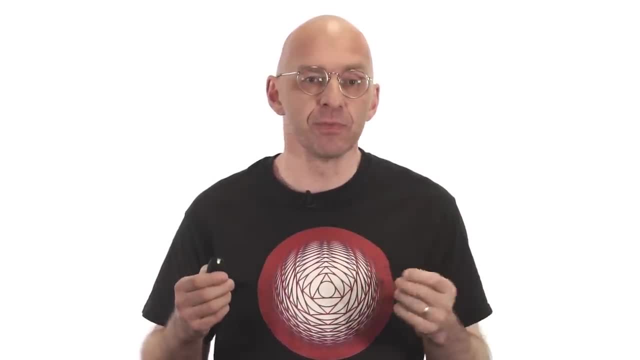 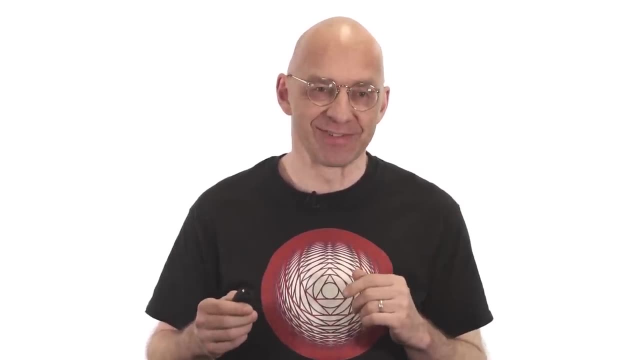 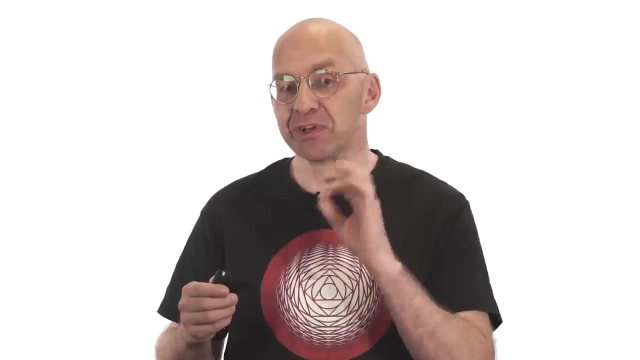 these impossibility proofs, Not many people, except a few pure maths majors who may encounter them, immersed in a course on Galois theory- Really heavy duty stuff. However, on close inspection it turns out that those proofs only really require some of the semi heavy-duty parts of Galois theory. Then if 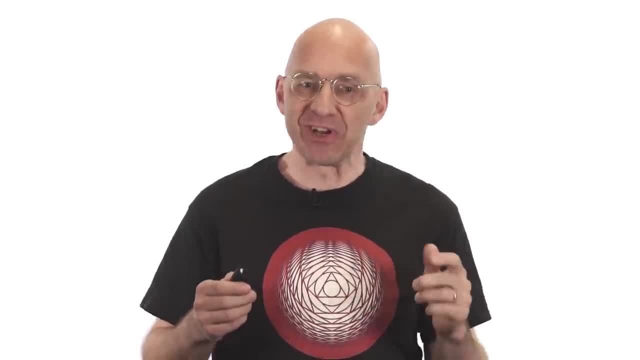 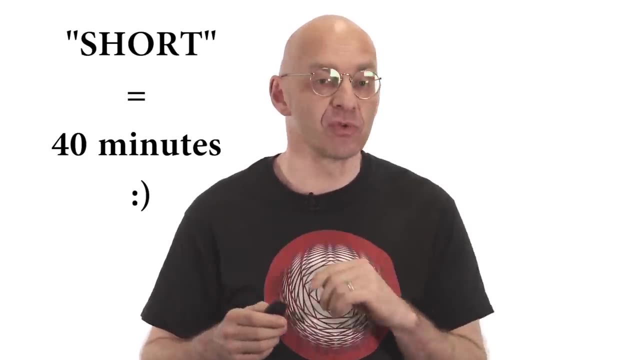 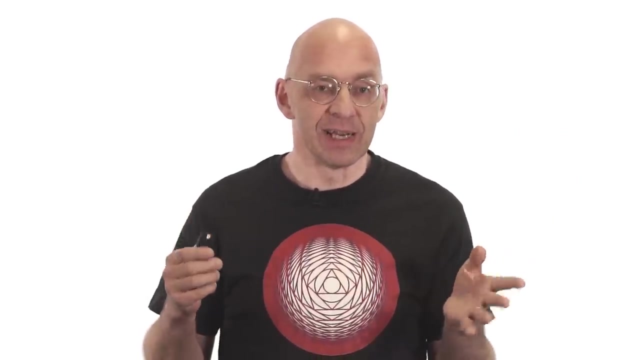 you are incredibly stubborn and you try really, really hard. it's possibly possible to distill the essence of these proofs into one short and not too hard YouTube video. I don't know about you, but I find the idea of making a video like this super exciting. It's an opportunity to make a small but. 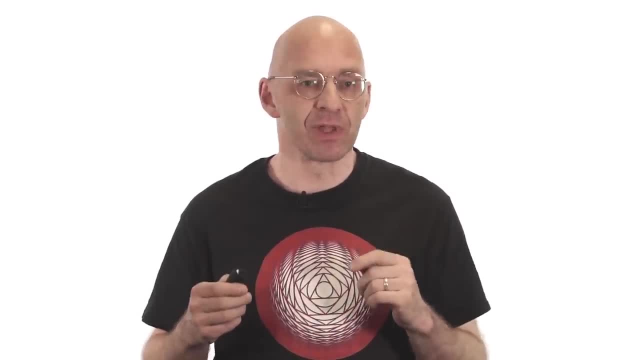 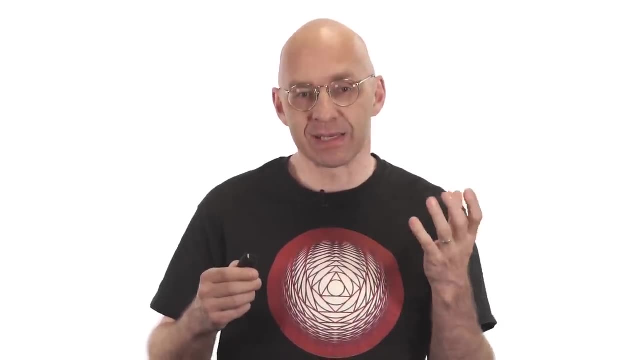 tangible contribution to something that people have been struggling with for thousands of years, And I hope that for you it's an opportunity to get to the core of some classic and beautiful and hard mathematics To get some insight into a few of these proofs. And I hope that for you it's an opportunity to get to the core of some classic and beautiful and hard mathematics To get some insight into. 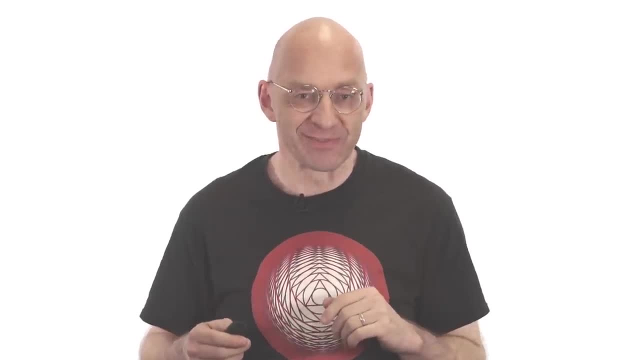 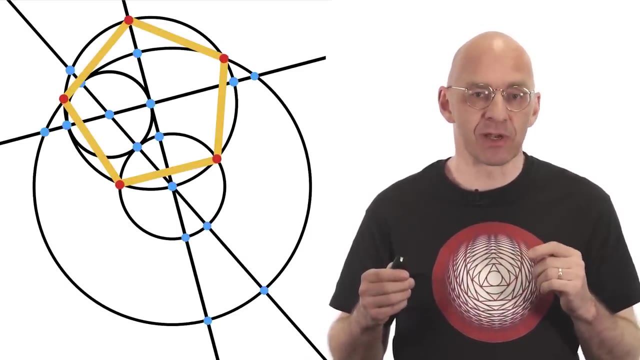 a theory normally considered out of reach of mere mortals. Okay, here's the plan for today. I'll first tell you exactly what it means to construct things with rule and compass the precise rules of the game. Then I'll go very carefully through. 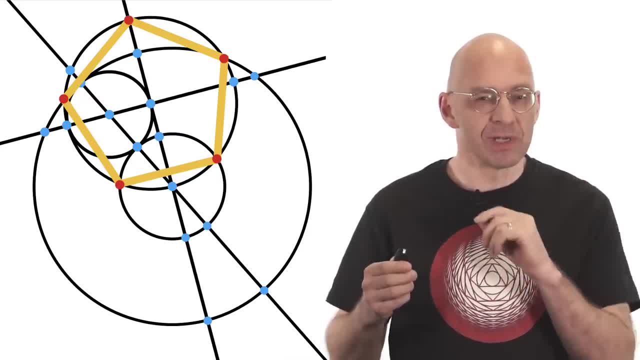 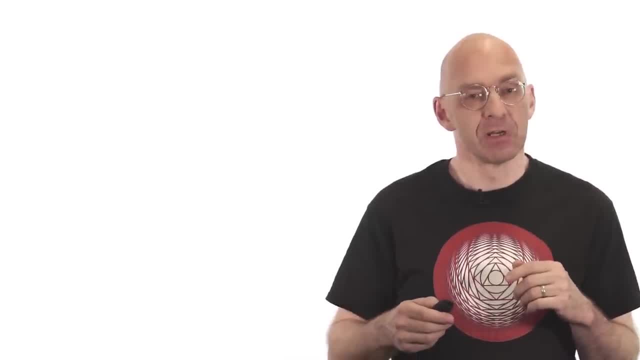 the proof that doubling the cube is impossible. Our argument that doubling the cube is impossible will be a proof by contradiction and will run like this: If doubling the cube was impossible, then doubling the cube is impossible. If doubling the cube was impossible, then doubling the cube is impossible. If doubling the cube was. 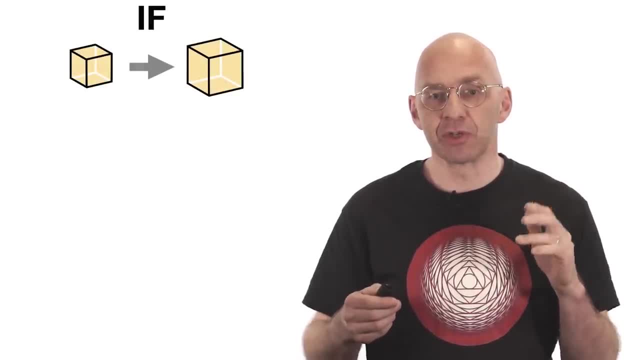 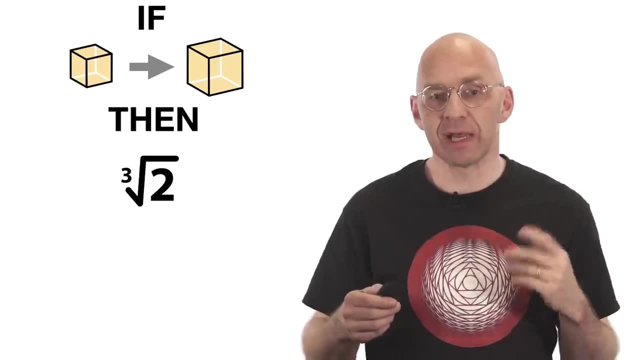 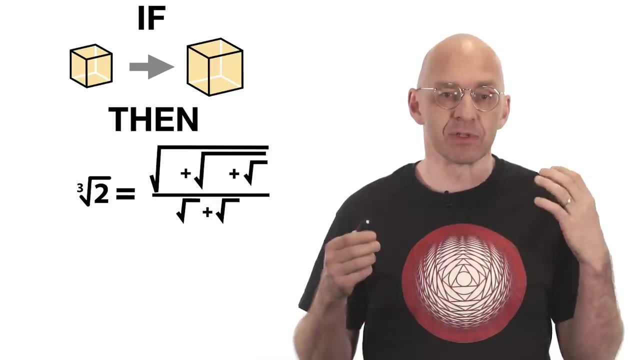 was possible, then we can use that to show that the cube root of two, a number closely related to our problem, could be written as an expression that only involves rational numbers and square roots. However, as will also show, this would imply that cube root of two is, in fact, equal to a rational number, Since 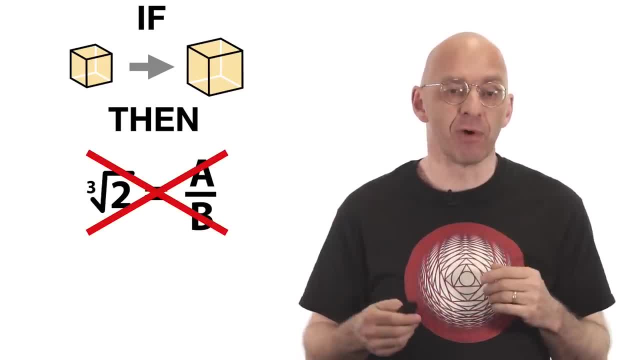 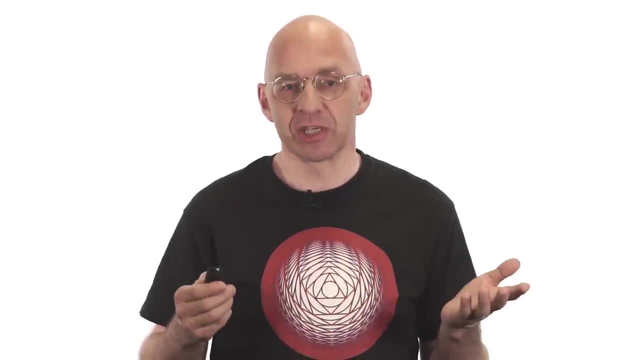 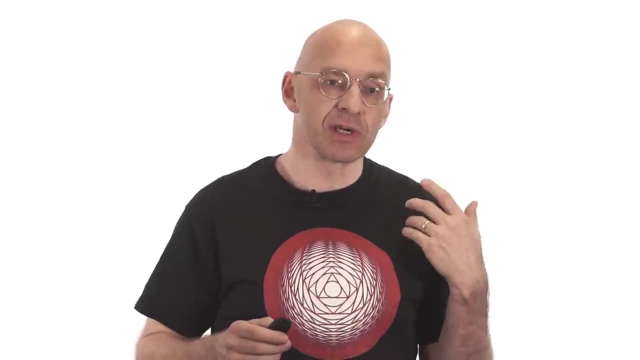 this is definitely not the case. doubling the cube cannot be possible either. After the hard work of doubling the cube, I'll then tidy up by sketching how this wonderful proof by contradiction can be modified to also take care of trisecting angles and constructing regular heptagons. And 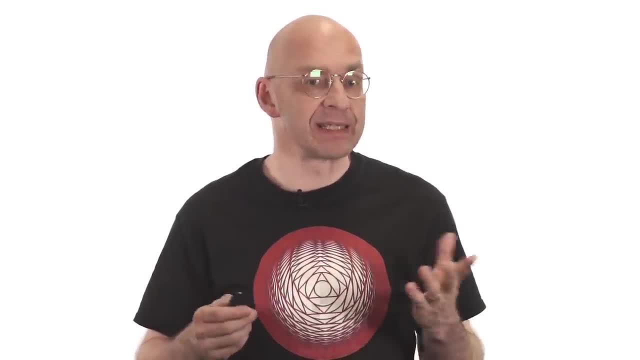 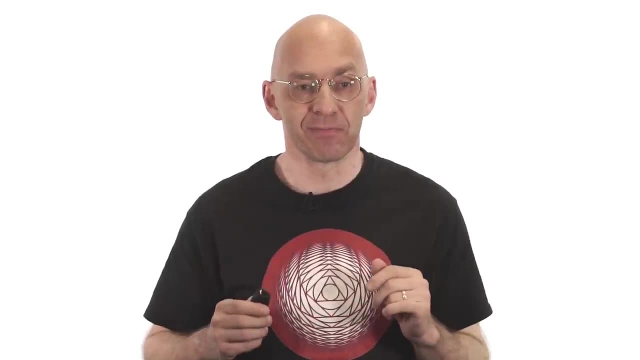 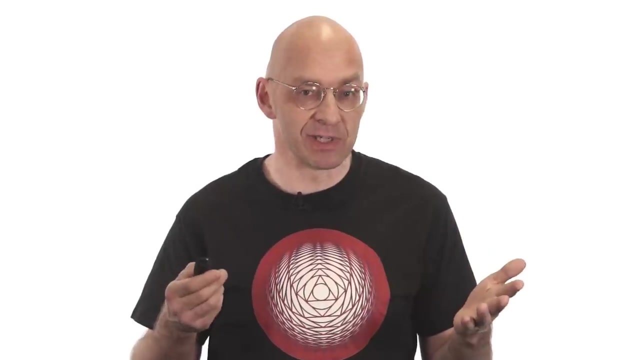 finally square in the circle can also be ticked off easily, because we already did most of the heavy lifting for the proof in a previous video on the transcendence of pi. As you may already have guessed, this video is a challenging one. so, as for my previous master class videos, this one is broken into levels of 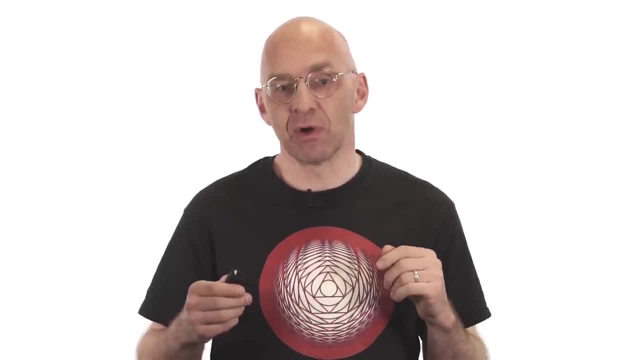 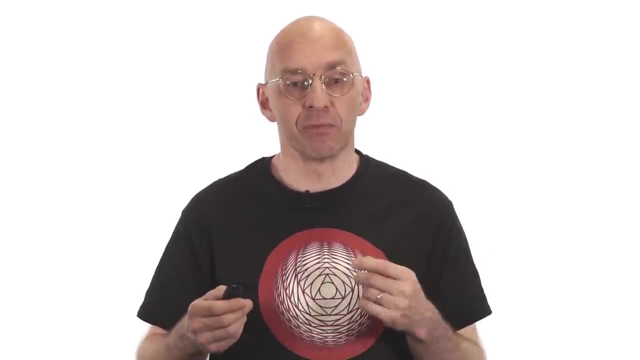 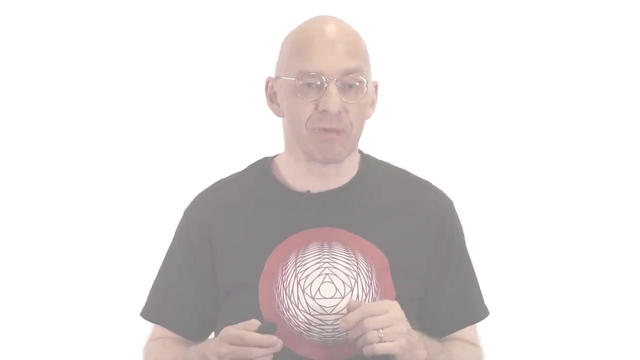 enlightenment. Six in all, and each with its own mathematical superhero guide. Of course, feel free to start skipping if it gets too tricky, and let me know how far you make it in the comments. Okay, without further ado, mathematical seatbelts on and on to level one. 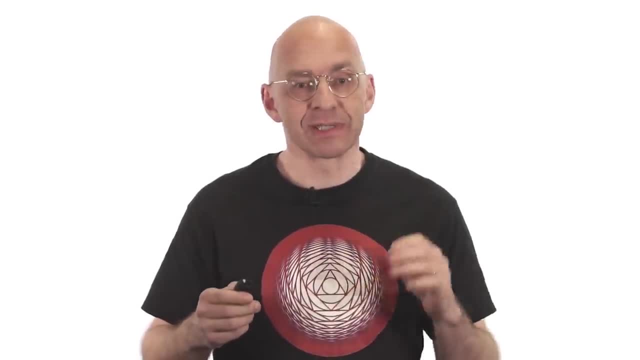 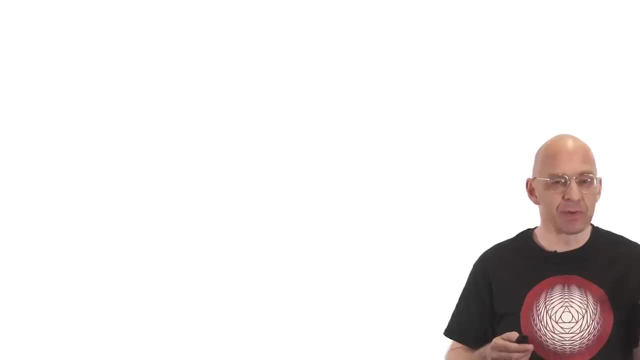 This video is all about the things that a ruler and compass cannot do. but first let's ask: what can they do? What can we construct with ruler and compass? To start, let me begin drawing to just give you a feel for what's going on. 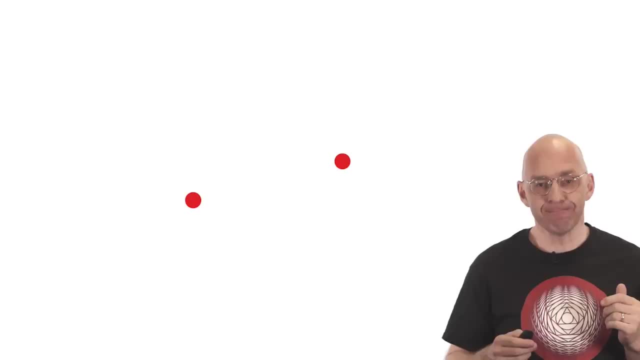 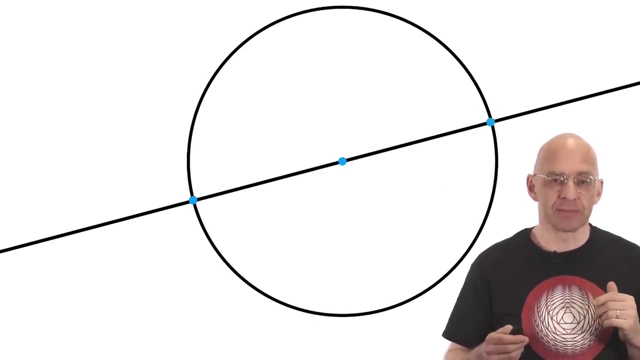 Okay, let's start with two points in the plane. Now draw the line through them. Okay, draw a circle with this red point as its center through the other point. So now we have a third point, the other spot where the circle and line intersect. Draw. 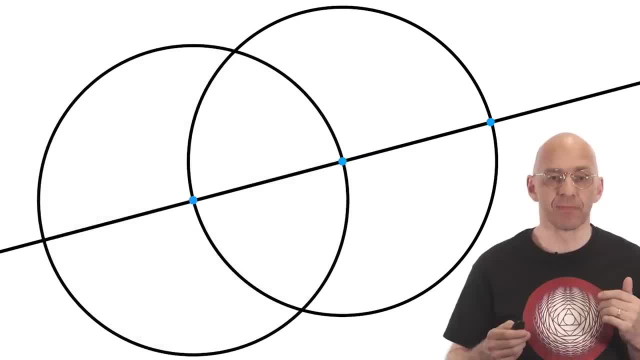 a center point as center through this new green point. That gives us three new points of intersection, and our construction is already getting pretty and also pretty interesting. Now draw a line connecting these two red points. another intersection: Clearly, this point is the midpoint between our two starting 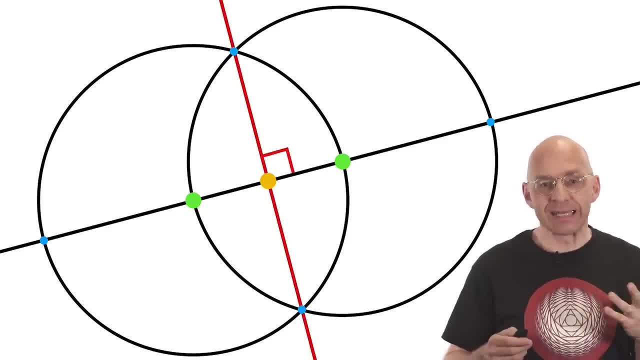 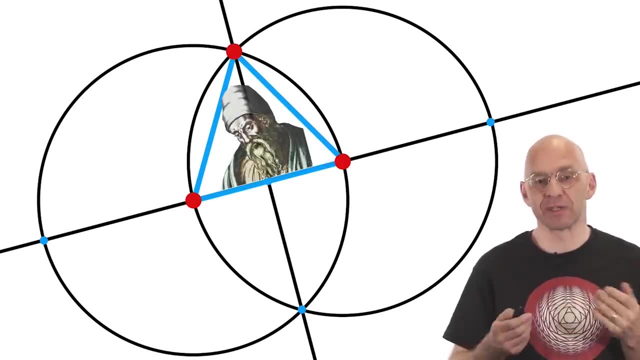 points, and our second line is clearly the perpendicular bisector of our starting points. Plus these three red points, there are the corners of an equilateral triangle. Pretty impressive. By just drawing a couple of lines and circles you get all this good stuff. What else is? 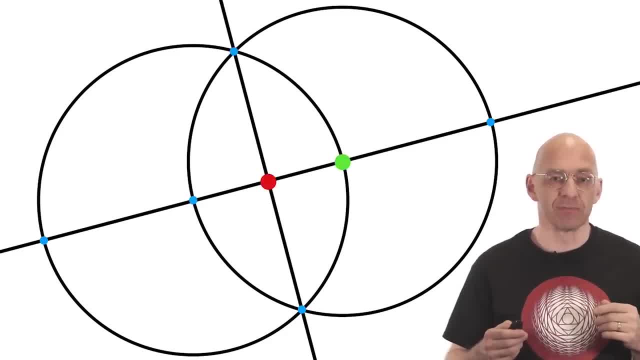 there, Let's draw another smaller circle like so: Okay, two more points of intersection which, together with the original two points, form the corners of a square. Pretty easy, right? A regular hexagon is also hiding just around the corner. Let's go and find that one too. 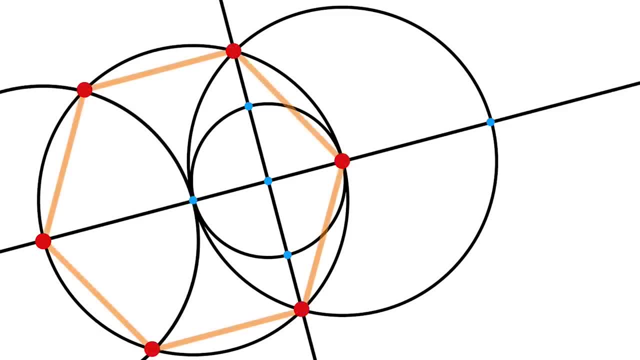 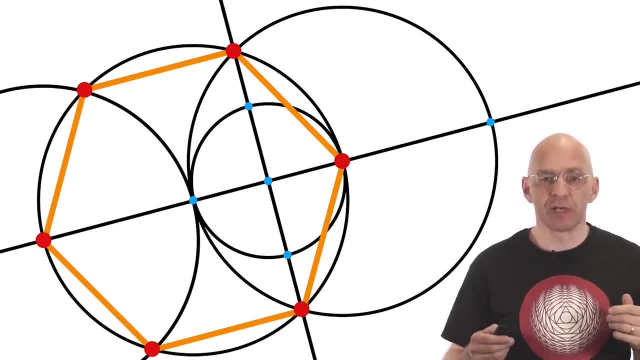 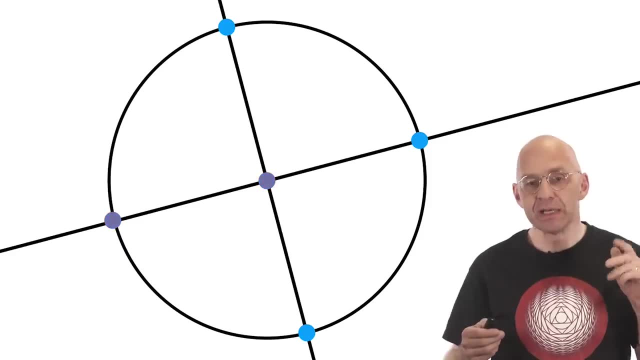 All child's play, but what about regular pentagons? That's not so obvious. Let me show you how you can do this, starting with this part of the picture There, just that one. First, we locate the point halfways between these two points. Now, 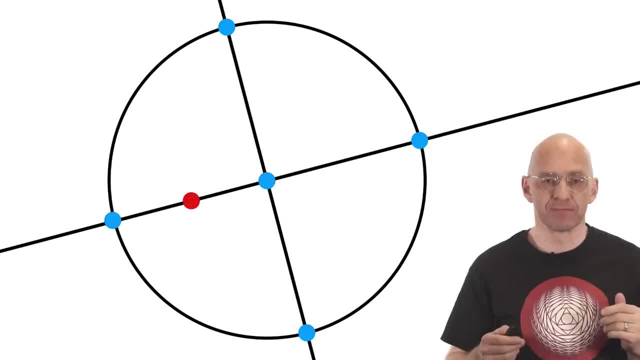 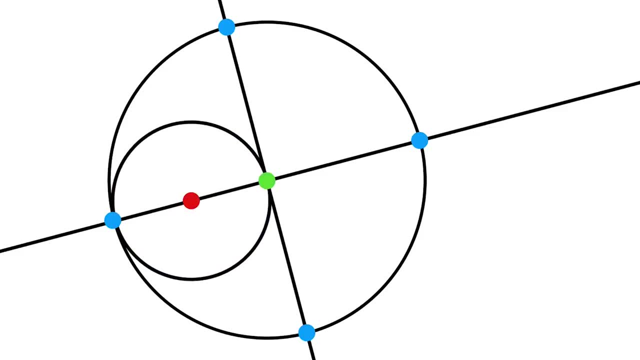 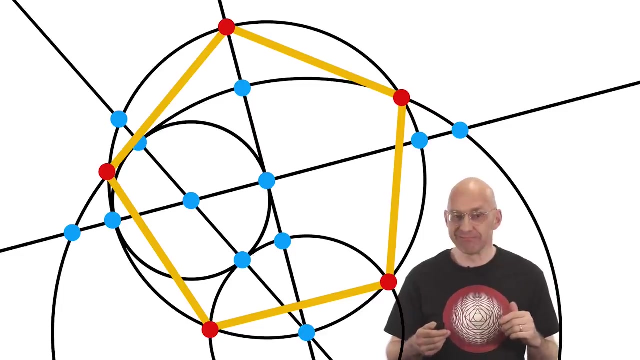 you all remember how to do that right, So I'll skip the details. Nothing very five-ish yet, but just watch. Pretty cool, right? But maybe I cheated. Is that really a perfect, regular pentagon? It definitely is not obvious, but yep, it is. And your first real challenge today is to 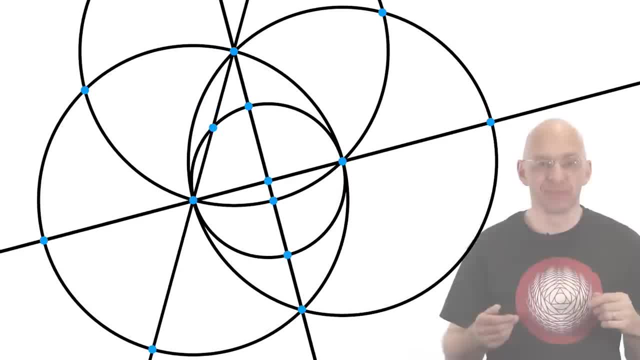 work through the details and nail down a proof. Okay, so, having played with ruler and compass a bit, we're ready to declare the rules of our game. Here we go. At any stage of the game, we have before us a collection of points, lines and circles. right, Then there are two ways we can. 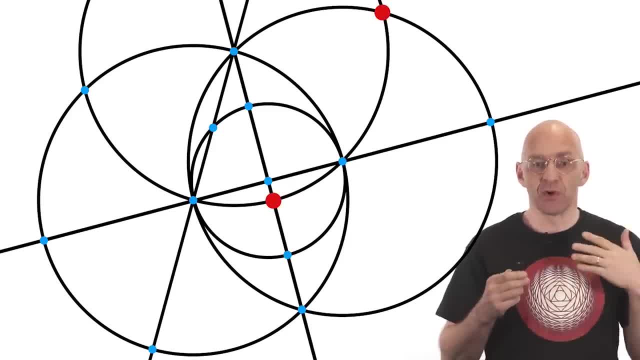 proceed First way: choose any two points and draw the line through them. As well as adding the new line to our collection, it also adds all the intersection points of this new line with the previous lines and circles. So let's go ahead and start. 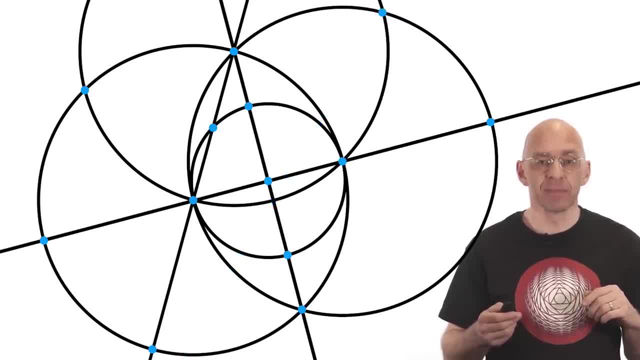 So there you go, all of those go in, and there's a second way, and that second way is to again start by picking any two points, and then you draw a circle centered at one of the points and passing through the second point. The new circle is then added to the collection, as are all the new intersection points. 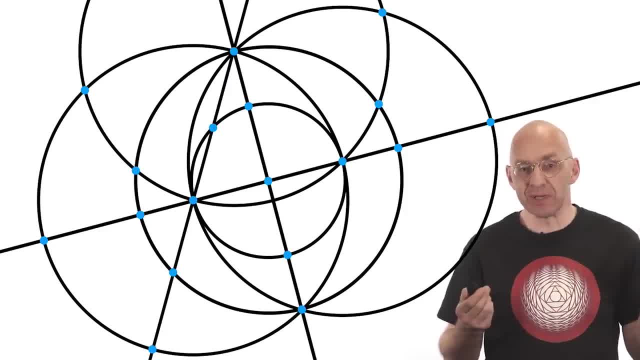 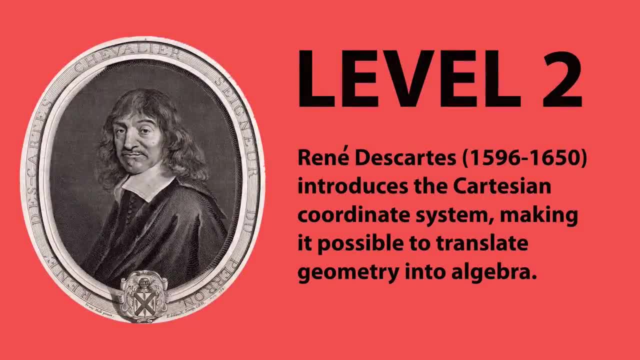 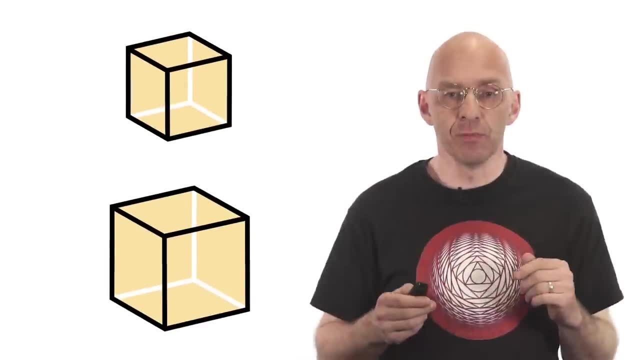 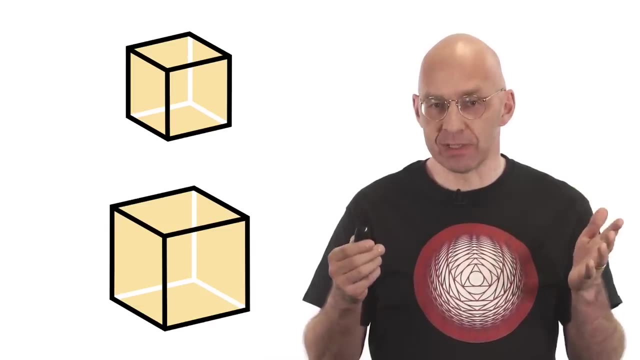 So those are the rules of our game. Pretty easy, right Now, what about those special problems, doubling the cube and so forth? Okay, you have a cube and your aim is to double its volume using just ruler and compass. What this means in our game is that you start with two points: the side, 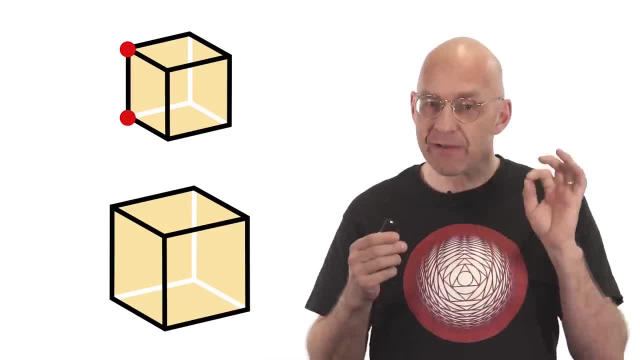 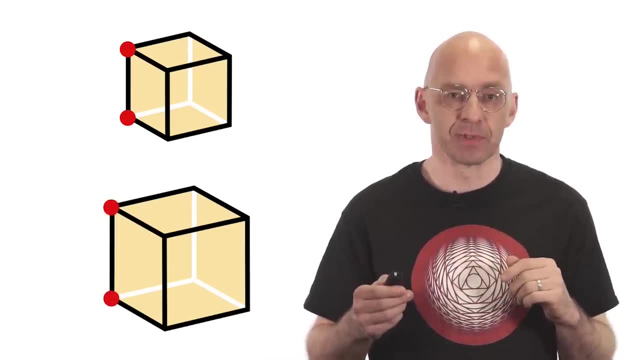 lengths of our cube apart, and your aim is to construct, in a finite number of ruler and compass steps, two points that are the side lengths of the double cube apart. For the purpose of this game, we're going to start with two points and then we're going to start with two points. For the purposes of our game, we can assume that our original cube has 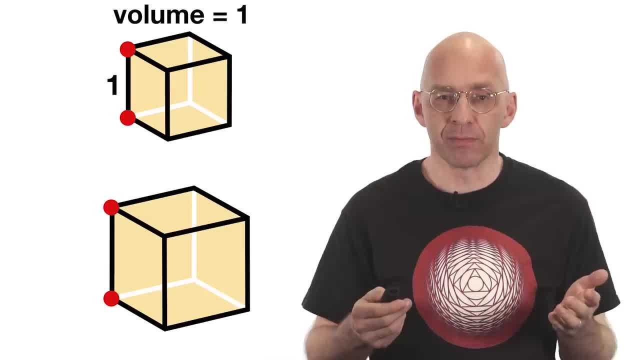 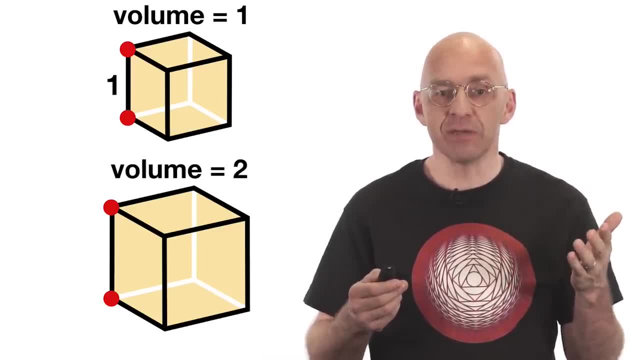 side lengths one, and so also volume of one, And the volume of the double cube would have to be two, of course, right, And so its side lengths would have to be the cube root of two. Got it Starting with two points a distance, one apart, our 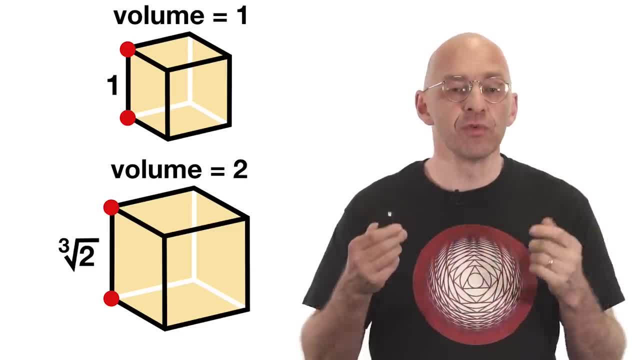 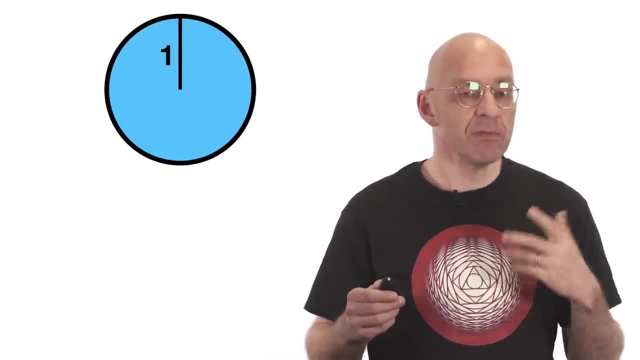 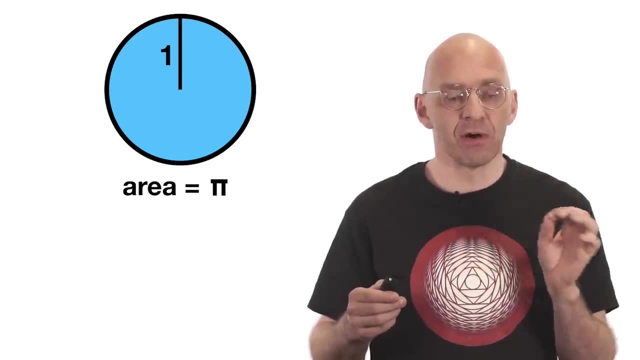 aim is to construct two points that are a distant cube root of two apart. Similarly, a circle of radius one has area pi, So constructing a square of the same area means the square should have a side length of root pi. As I already showed you, constructing squares is not a 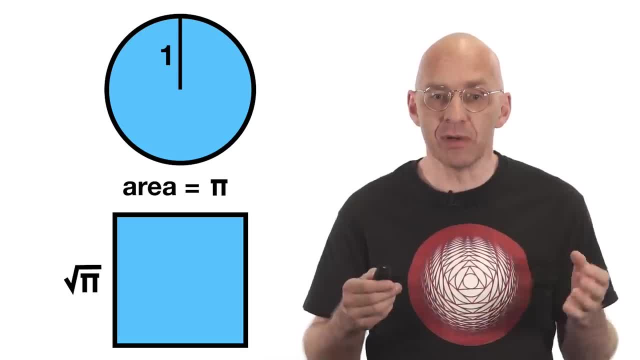 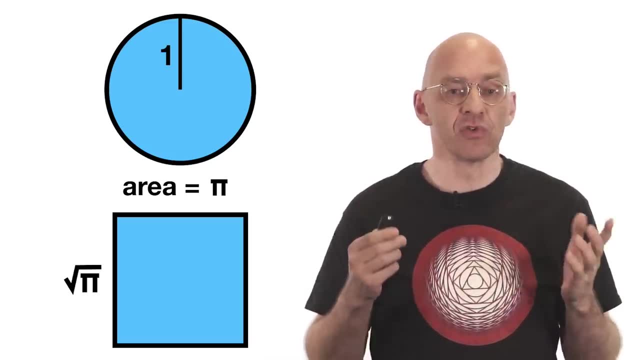 problem. so in our game, squaring the circle amounts to beginning with two points a distance one apart and using them to construct two new points a distance root pi apart, In exactly the same way. the other two problems I showed you at the beginning boil down to the following. 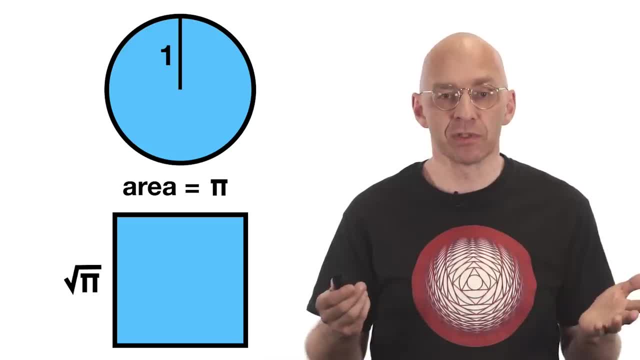 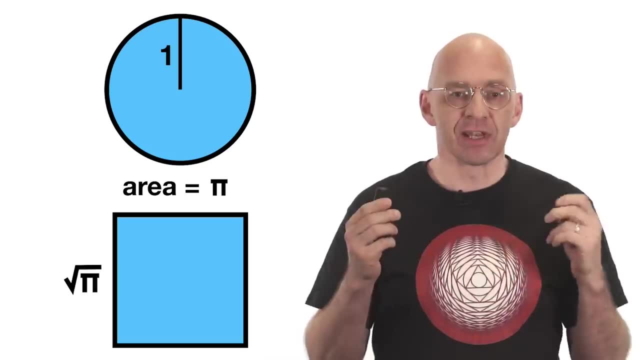 to starting again with points a distance one apart and using these points to construct two specific new lengths. In fact, let's go all cartesian and pin down things a little bit further. Let's make our two beginning points the origin and one zero, the point one unit to the right along the x-axis. 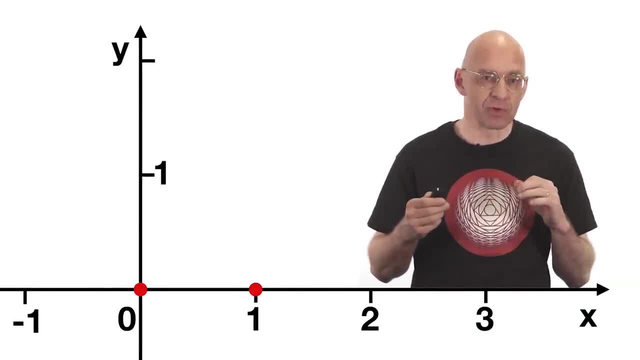 Now there's a little ruler and compass magic that I won't go into but which helps simplify our problems. It turns out that if we can construct a segment of a certain length somewhere, then we can always translate and rotate using ruler and compass to obtain a 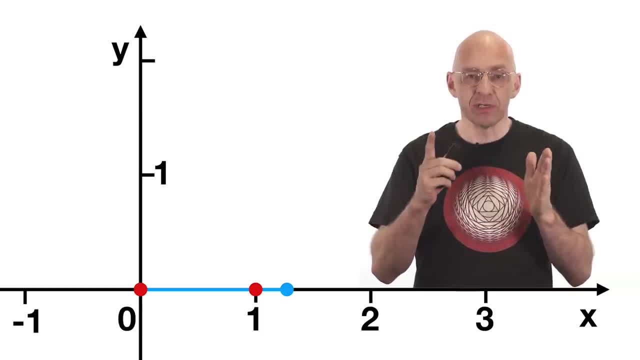 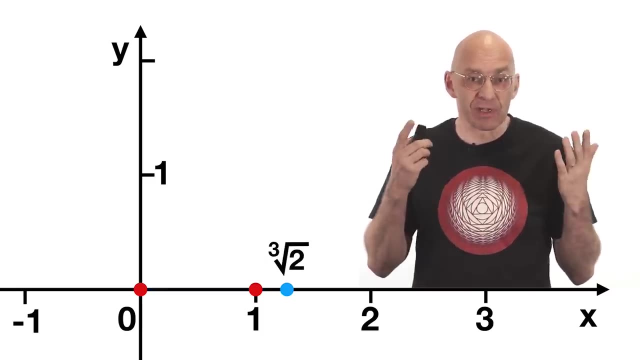 segment of the same length, starting at the origin and lying along the positive x-axis. That means our cube doubling problem boils down to using ruler and compass to locate the point- a distant cube root of two along the x-axis Similarly square in the circle boils. down to locate a segment of the unit beyond x-axis. We are still not sure why a ruler is so important in developing the problem, because it only salumes the following two Chronidd tales and in fact it directly discourages the answer to🎵 investigation of problems in this video. 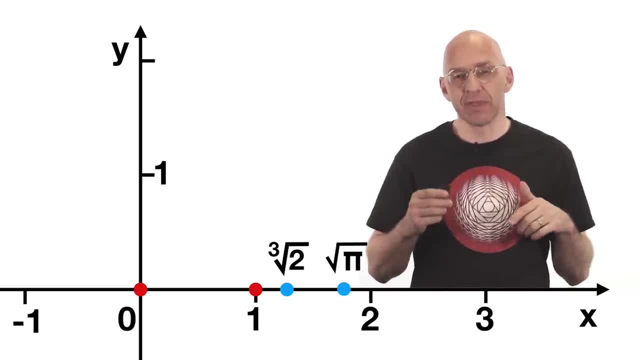 let's just see how we approach our problem. Let's have a beginning point and, to start with a link, root pi on the x-axis And there are two more mysterious numbers which arise from our other two problems. Those two guys, Of course, faced with the task of 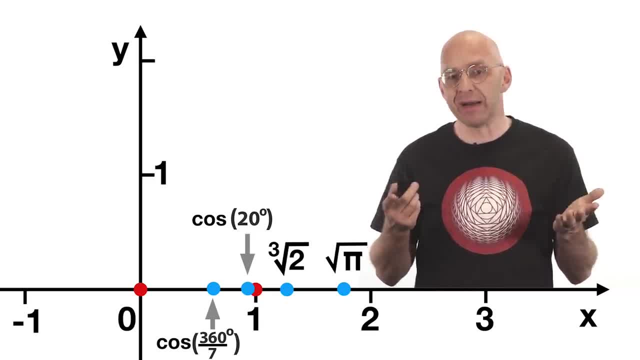 constructing numbers such as the cube root of 2 and root pi, it's natural to just stare helplessly into space, which is pretty much all that happened for 2,000 years. So let's look at it another way. Let's ask: what numbers can we? 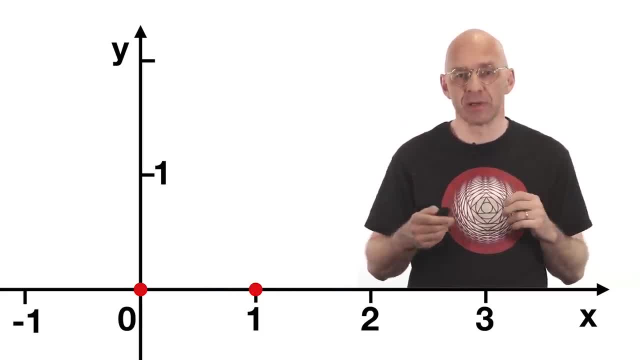 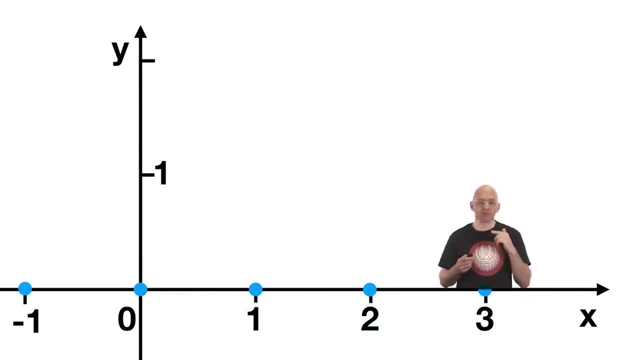 construct. Well, obviously all the integers can be constructed like this. Then, as we've seen, we can construct midpoints. These are the integer multiples of 1 half. They are mob midpoints here. This gives all the integer multiples of 1, fourth and so on. What else? 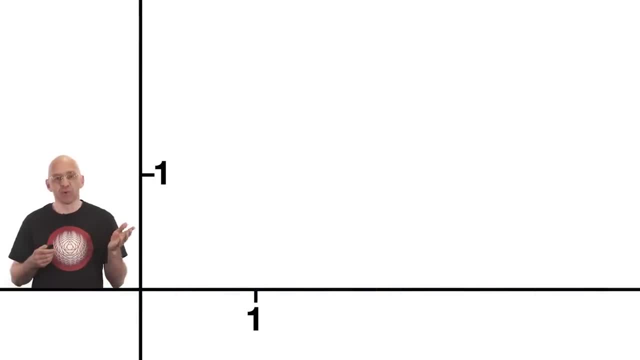 Lots. It turns out that once you've constructed two numbers, a and b, you can also construct their sum, their difference, their product and their quotient by executing four easy constructions. For example, to construct a plus b, you just need to transfer distance, which, remember, is no problem with ruler and compass. So 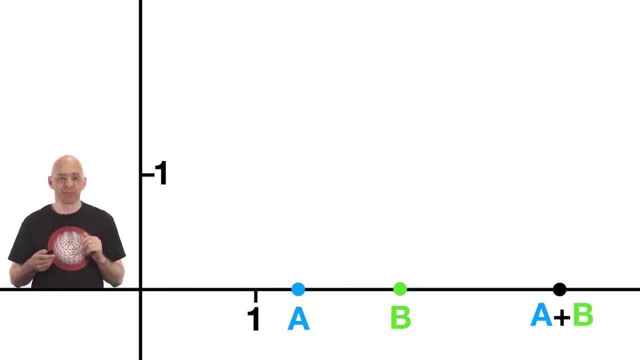 there we go, Just push it over and that's a plus b There, And b minus a is just as easy. Okay, let's have a look. Let's push this over. That's b minus a. Next, to construct a times b, we also need to be able to construct perpendiculars, which we've 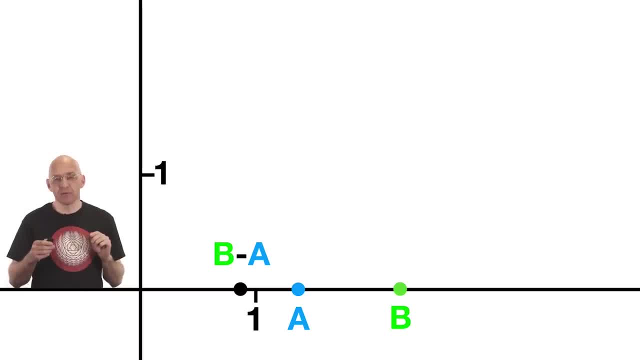 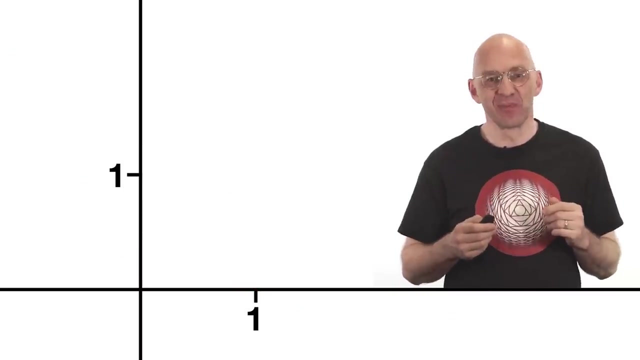 already seen, and to draw parallel lines, which is also straightforward with ruler and compass, Ignoring the fiddly details, here is the key idea of this product: construction- Pretty nice, huh. And constructing a over b is similarly easy, Fantastic. Okay, so we can add, subtract, multiply and divide constructible numbers. 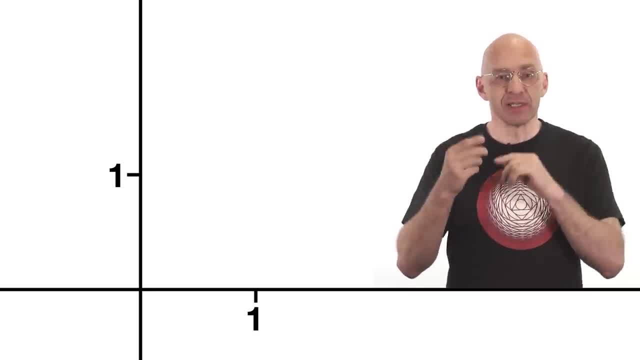 and with the integers already constructed. this means that all quotients of integers are constructible. In other words, we can construct all rational numbers with ruler and compass Anything else. We can definitely construct some irrational numbers. For example, root 2 is the diagonal of a unit square, which is easy to construct, In fact with a little. 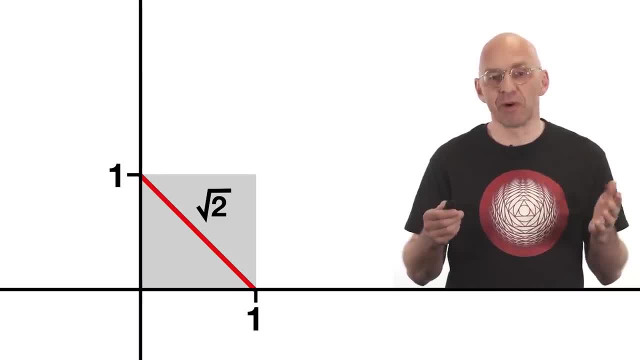 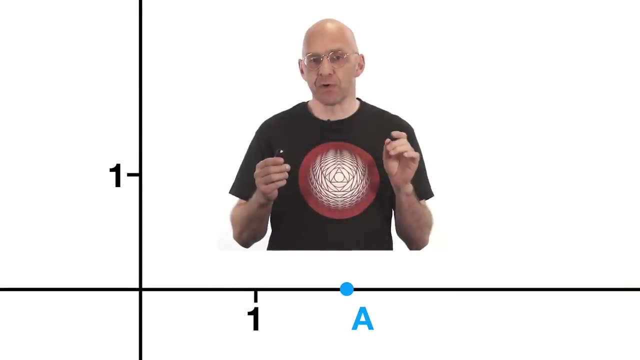 Pythagoras-ing. it's easy to construct the square root of any positive integer, But there's more. I'll now show you how, taking any positive number we've already constructed, we can always construct that number's square root. Suppose we've already constructed the number a down there. 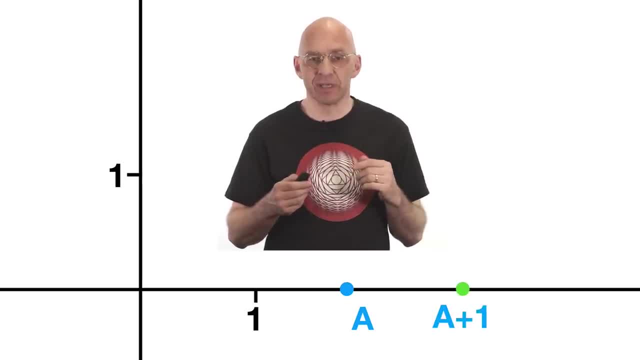 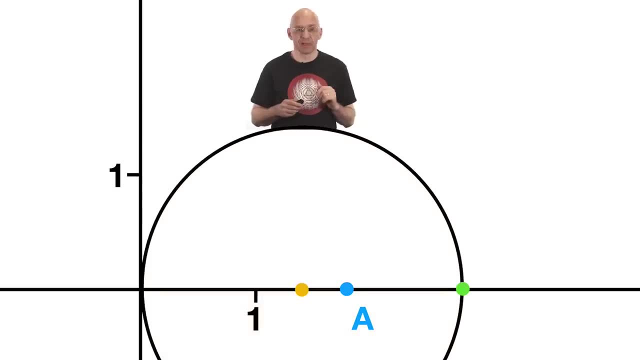 First at 1 to a, to get the green number here using rule and compass, of course. Now half the green number, draw this circle, draw the perpendicular through the blue point, then the pink segment has length root a. A pretty easy recipe to follow. I'll leave it as homework for you and your friend Pythagoras. 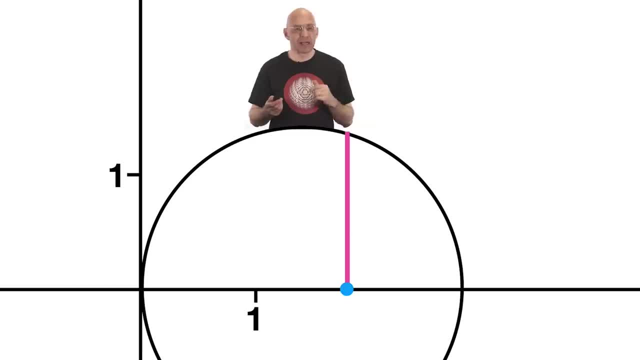 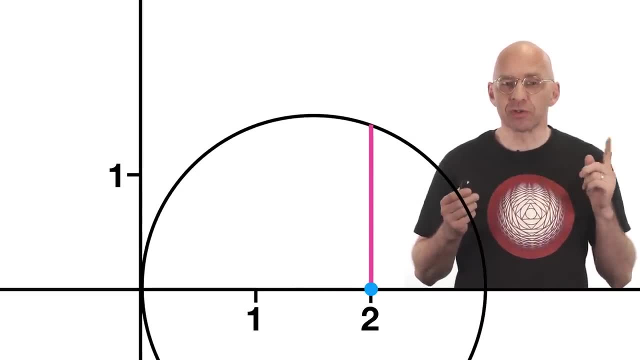 to check out that this actually works. But just for fun, let's calculate root 2 this way. That should be root 2, but root 2 is also the length of the diagonal of a unit square. There's the square. Well, let's check. Yep, that looks about right, which means it must be true. 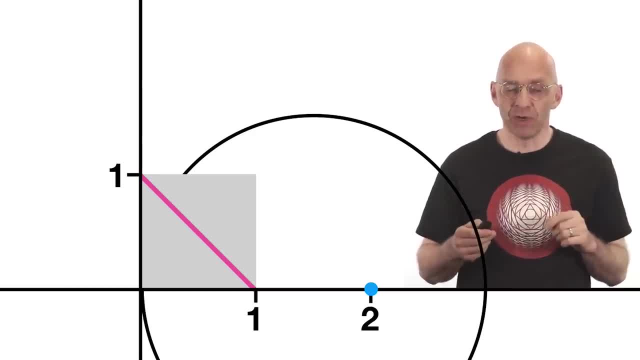 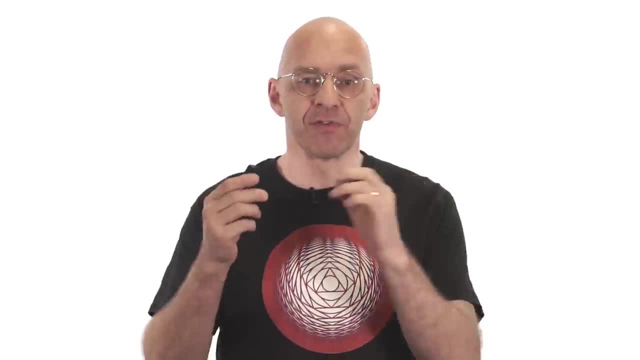 Well, of course not, But as you will show in your homework, it is right, Right, Right, You will show this. So it turns out: we can construct a lot of numbers, Starting with the numbers 0 and 1. we can add, subtract, multiply, divide and square root. 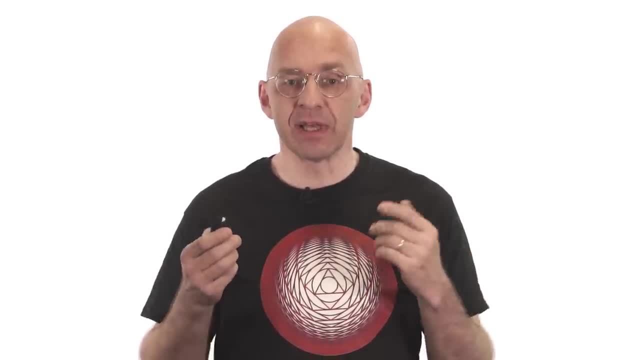 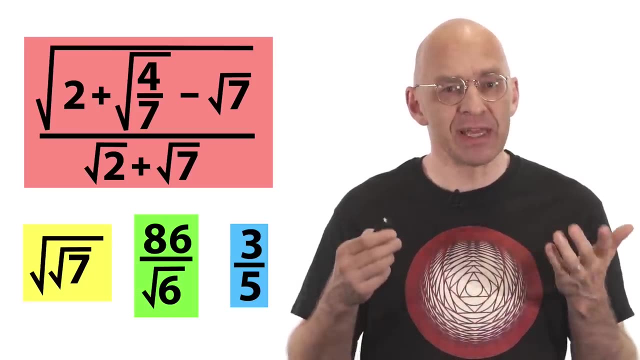 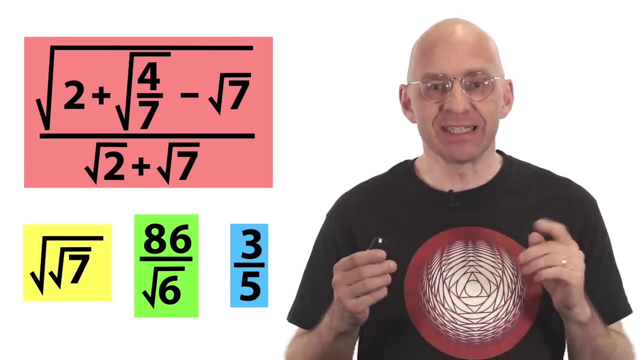 length any finite number of times. And here, then, are just a few examples of numbers we can construct. That's a ton of constructable numbers, but are there even more? What do you think? The answer to this question is no. These nested square rooty creatures based upon the 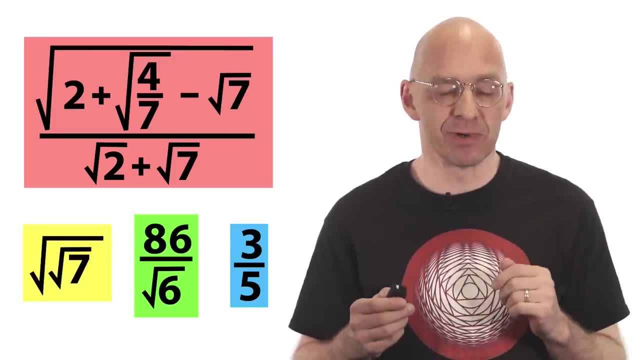 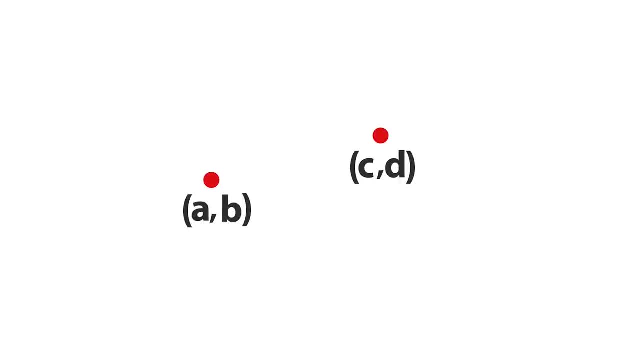 integers are the only kind of numbers we can construct with rule and compass, And it's actually very easy to see that this is the case. Suppose you have two points with square rooty coordinates, Then the equation of the line through those points will have square rooty coefficients. They're pretty 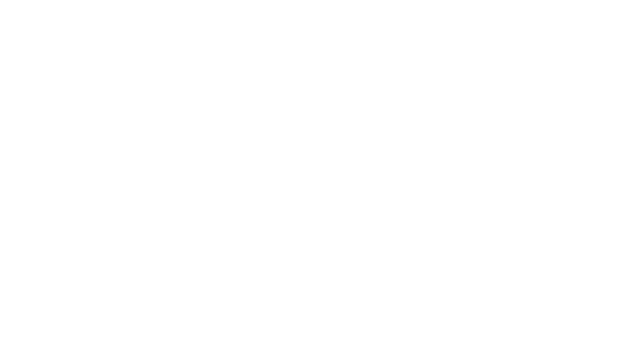 obvious. those are square rooty right, And a circle with square rooty center and passing through a square rooty point will have a square rooty radius, and so we'll also have an equation with square rooty coefficients There. that's the 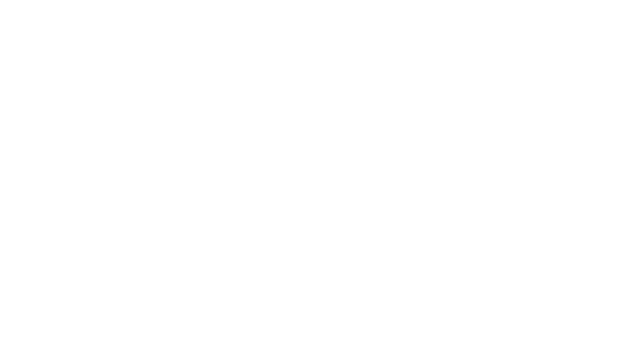 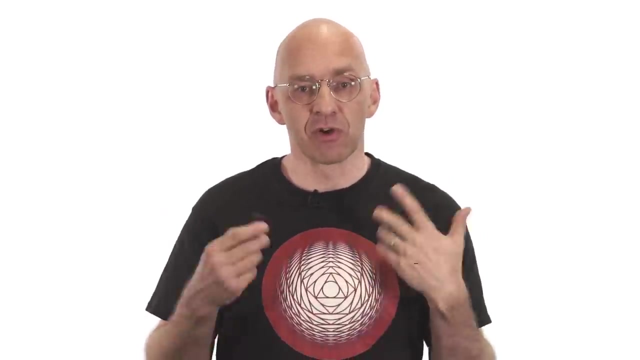 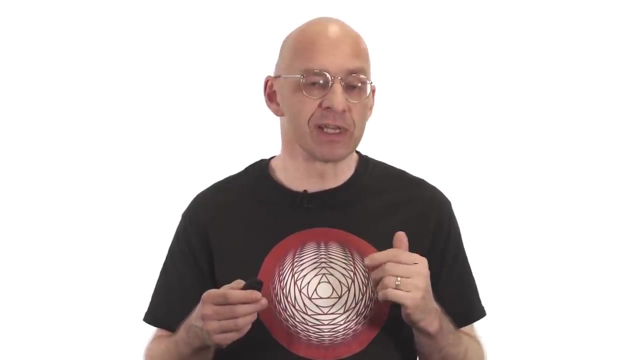 equation. And then how do we get new points? By intersecting lines with lines, lines with circles and circles with circles. That corresponds to solving pairs of linear and quadratic equations, and the solutions of those systems of equations are, of course, all square rooty again. And so, to summarize, start with our two. 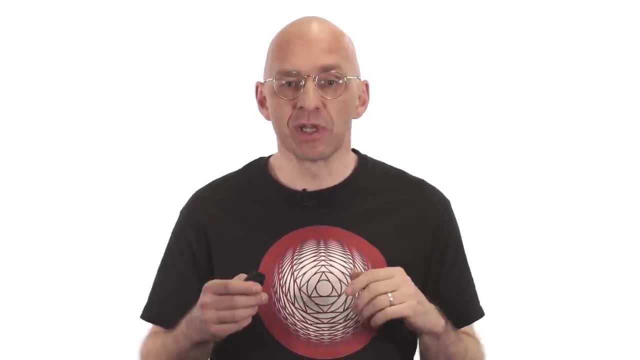 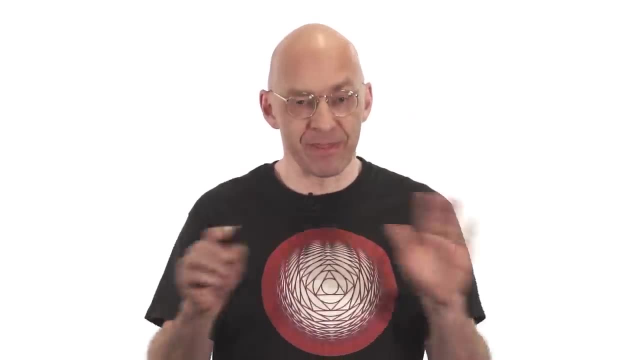 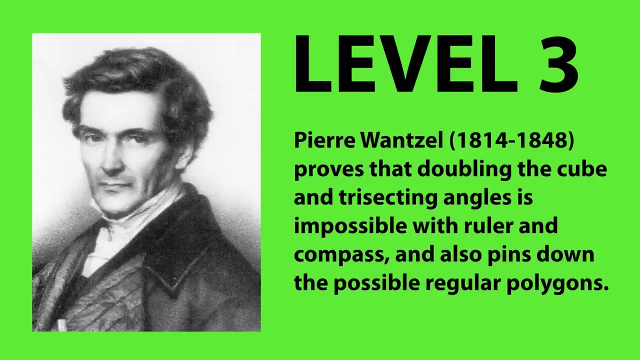 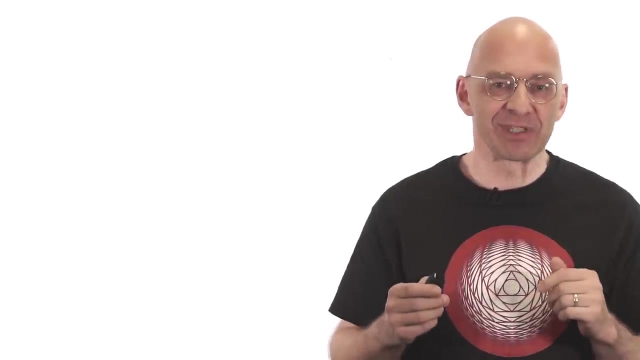 numbers 0 and 1 on the x-axis. We can use rule and compass to produce any square rooty coordinates we want, but only square rooty coordinates, nothing else. you So you're back for more. very good, So now we know exactly what type of numbers we can. 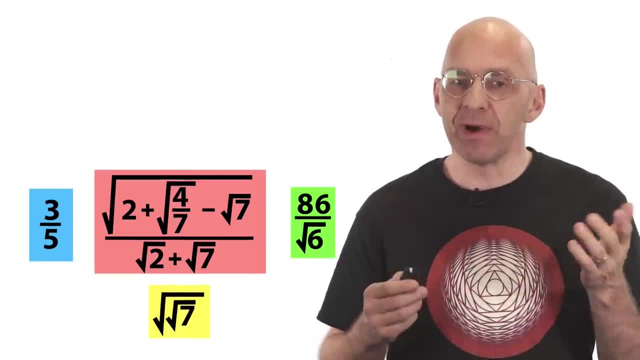 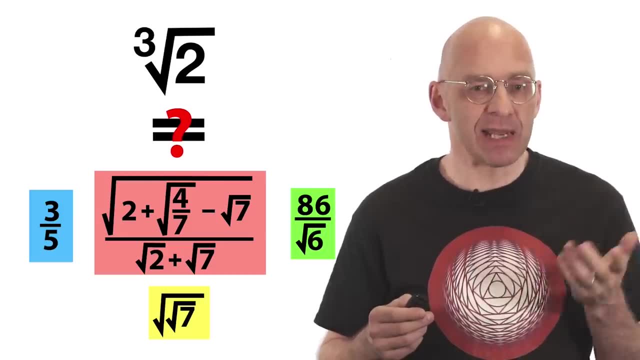 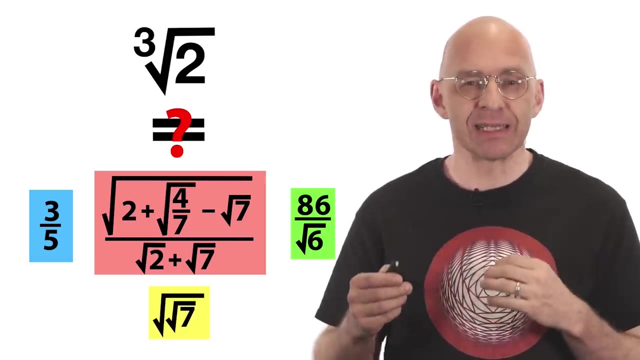 construct those square rooty monsters. but what about the cube root of 2?? Can that number be written as a mass of square roots? It seems unlikely, but how do we go about proving it? Well, some of those square root monsters are more monstrous than others, right? So let's start easy. consider some of the less. 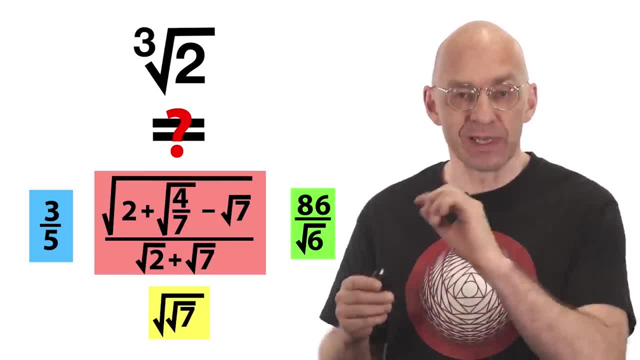 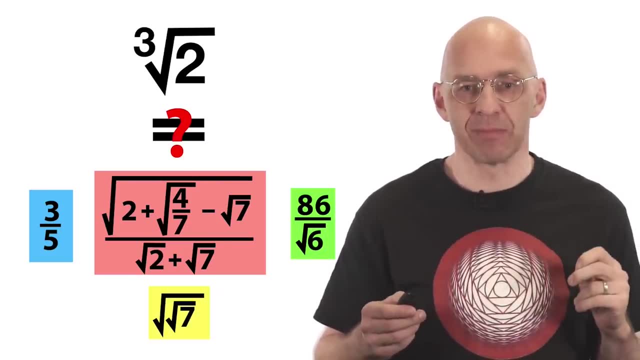 scary monsters first and work our way up. Hopefully we'll detect a pattern which will suggest the plan of attack. So what are the very simplest square rooty numbers? Well, that would be the fractions with no roots at all. So let's first ask: 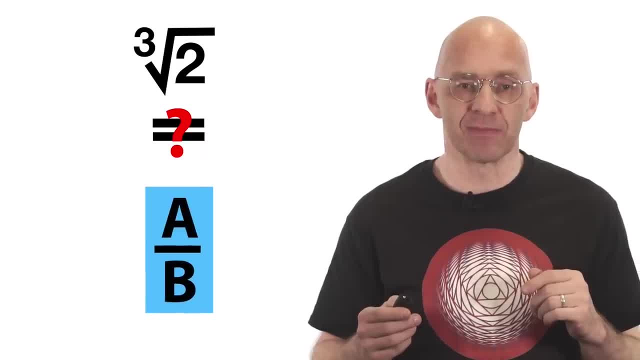 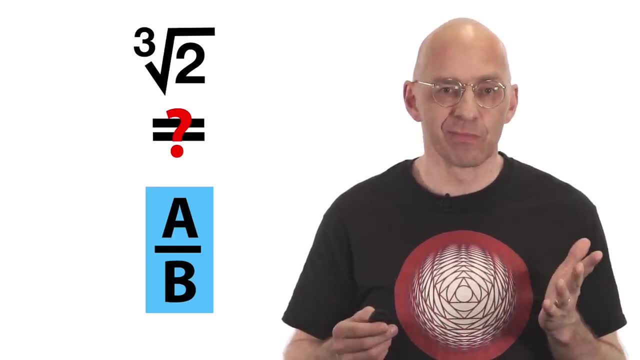 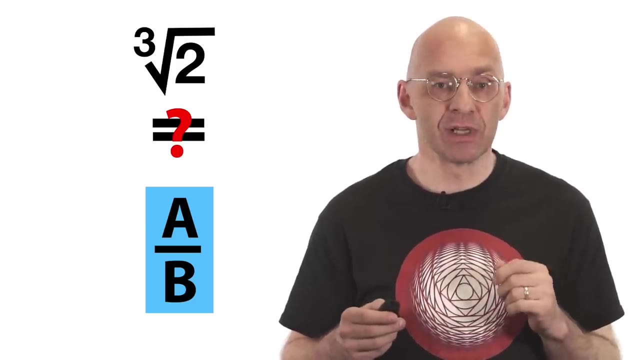 whether the cube root of 2 can be written as a fraction. That is our base level question is: is cube root of 2 a rational number? And, as all regular mathologer would know, the answer is a big no. The cube root of 2. 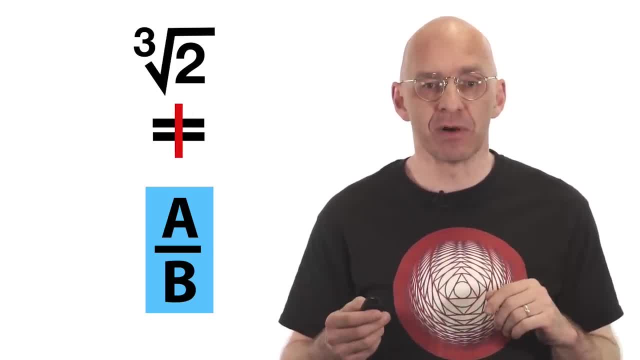 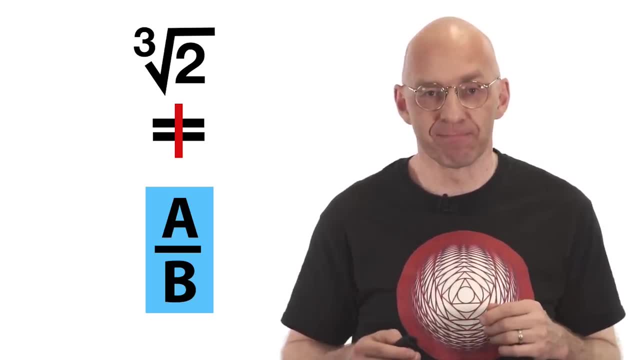 is not a rational number. I recently did a whole video about how you can quickly prove the irrationality of this and a bunch of other rooty numbers using the amazing rational root theorem. So let's take the irrationality of the cube root of 2 as a given. We'll also 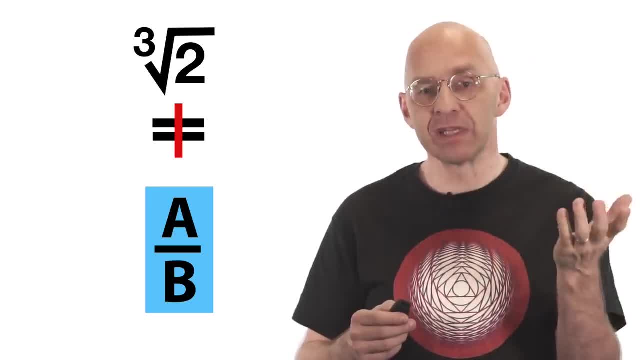 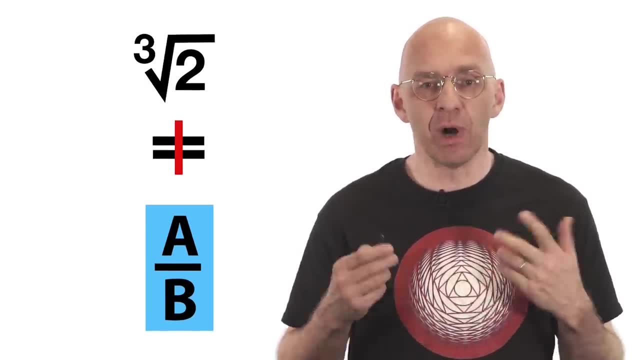 take it as known that square root of 2, square root of 3, square root of 5 and so on are all irrational. okay, Not a big deal. So let's take the irrationality of the cube root of 2.. Not a big deal. Okay. now as a warm-up exercise, let's think about all square. 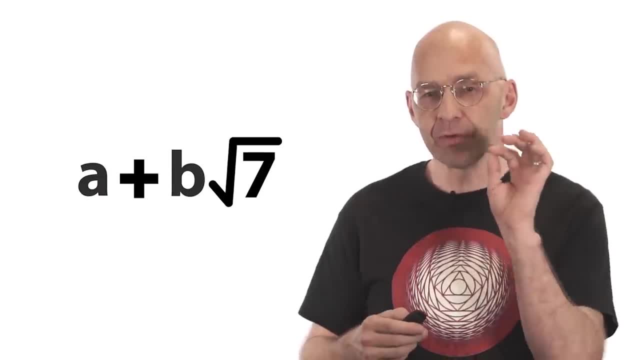 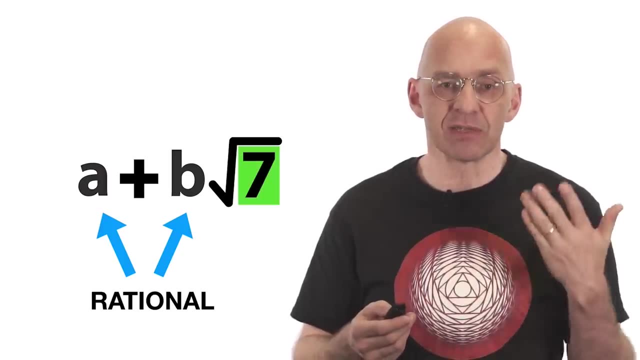 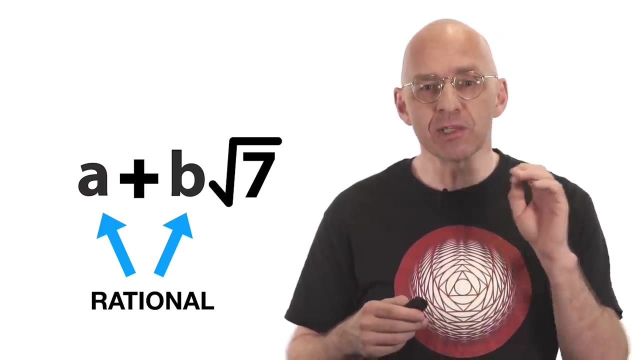 rooty numbers of this form there, where both a and b are rational numbers. There's absolutely nothing special about 7 here, just that it's a rational number whose square root is irrational. Could have used lots of other numbers there. Now, what we'd like to prove is that the cube root of 2 cannot be written as one of. 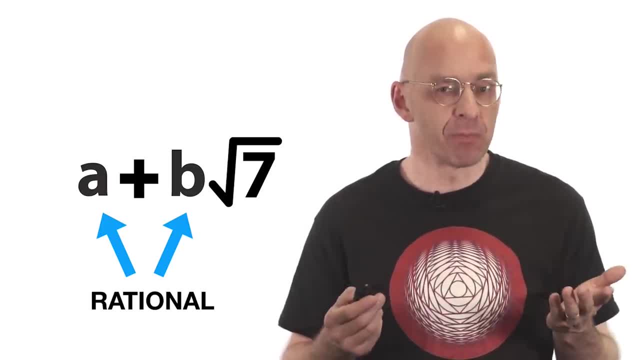 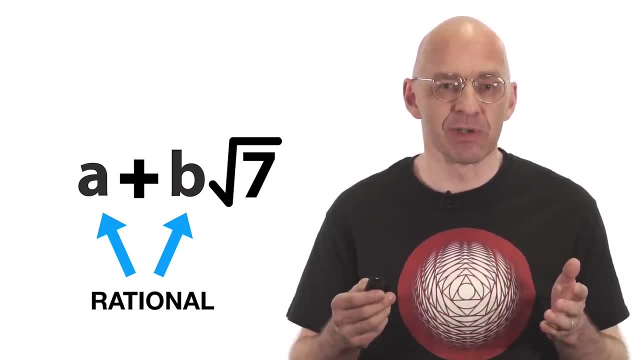 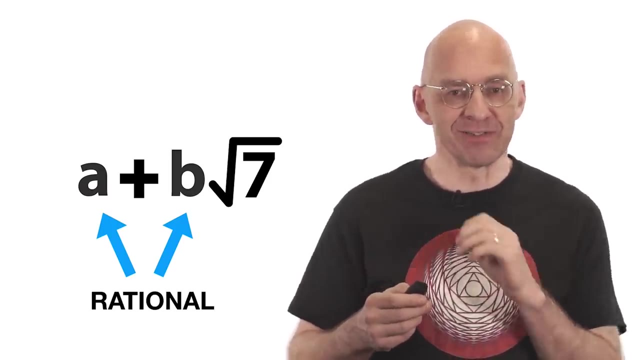 those root 70 numbers over there, That would be progress, right? Little tiny, special progress, but progress Now. if you're worried that this tiny progress will be too tiny, don't. Later there will be a humongous plot revelation that will more than compensate for the insi-vinciness here. Anyway, to prove, 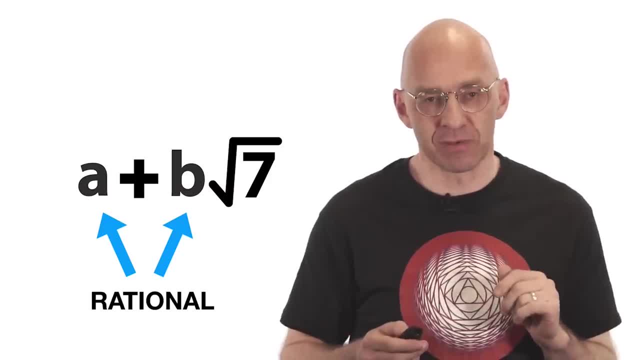 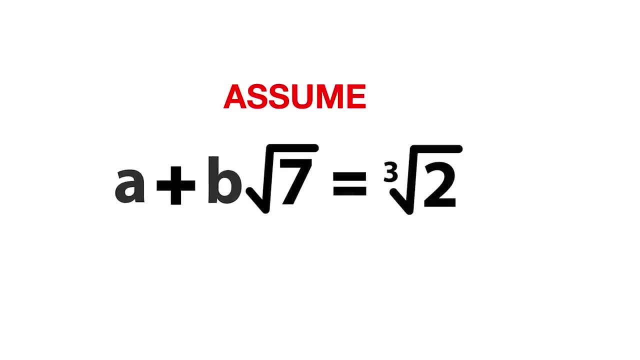 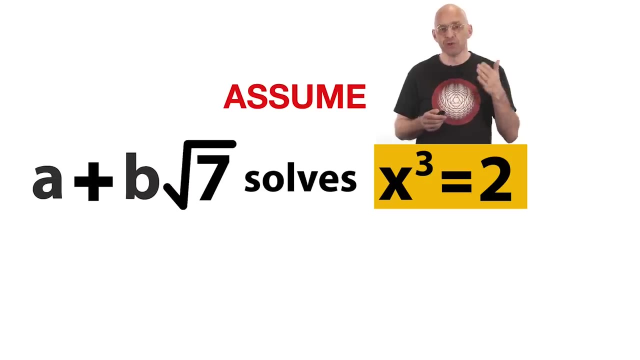 our special case, we set up the usual proof by contradiction. So we start by assuming that cube root of 2 is equal to one of these special numbers. In other words, we are assuming that our number is the solution of this equation here, Cubing the cube root of 2. 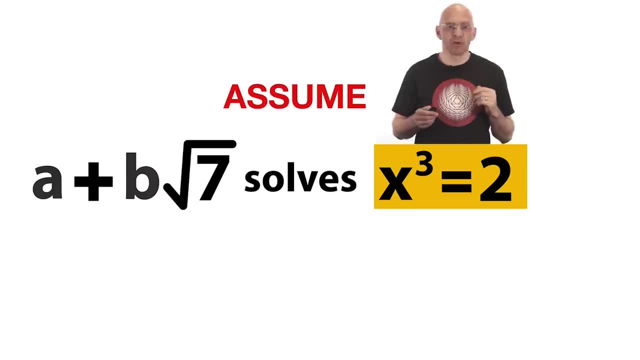 gives 2, right. In a moment we'll show that the assumption that a plus b root 7 solves the equation implies that the conjugate of this number, a minus b root 7, does so as well. However, ignoring complex number possibilities, this: 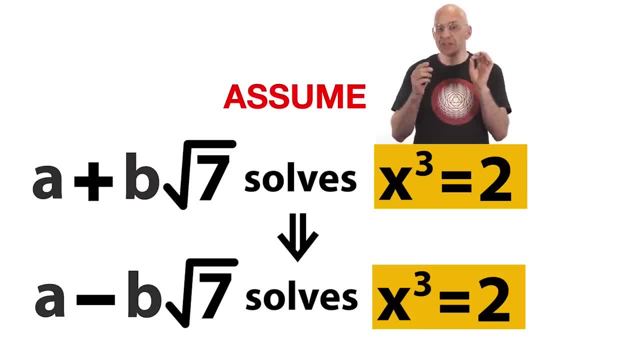 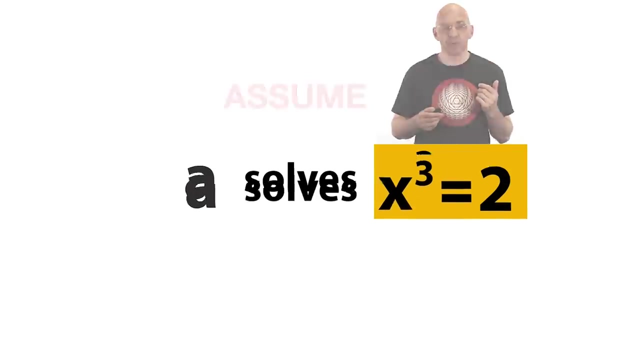 equation has one and just one solution: The cube root of 2.. Which means that our plus solution and our minus solution must be the same And b must therefore be 0. But that would mean that the root 7 stuff is irrelevant and that the rational number a itself would solve our equation, In other words the conclusion. 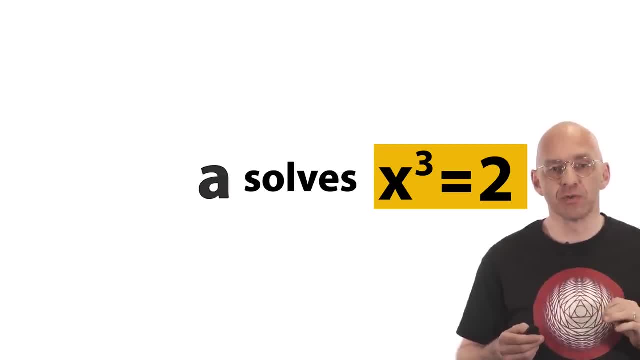 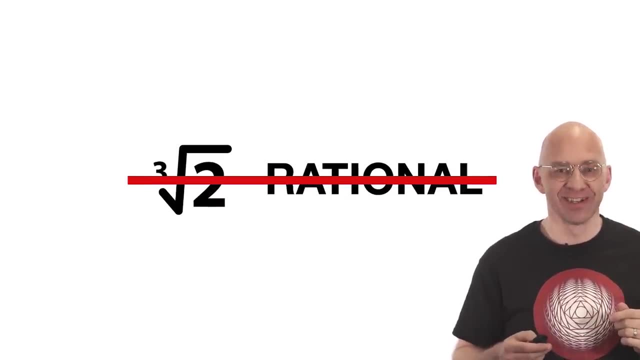 at the end of this chain of consequences is that cube root of 2 would have to be rational, Which, as you agreed, you agreed- is nonsense And therefore we've arrived at the contradiction we are chasing. So again, the assumption that cube root of 2 is of the form a plus b root. 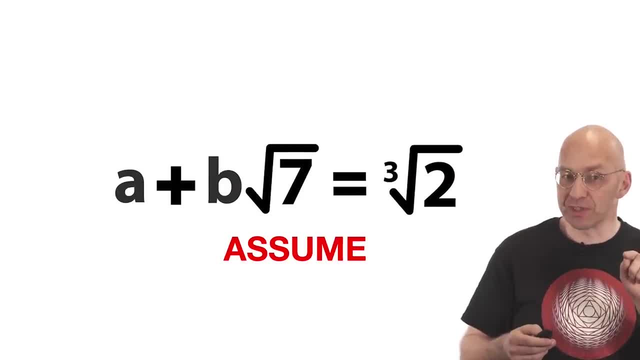 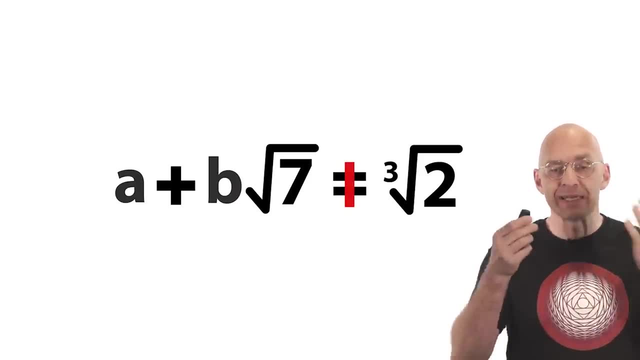 7 implies a contradiction which proves that the cube root of 2 is not of this form. But of course, to make the proof complete, I still have to fill in that crucial step of the argument. I have to show that if a plus b root 7 is of the form a plus b root 7, then the answer: 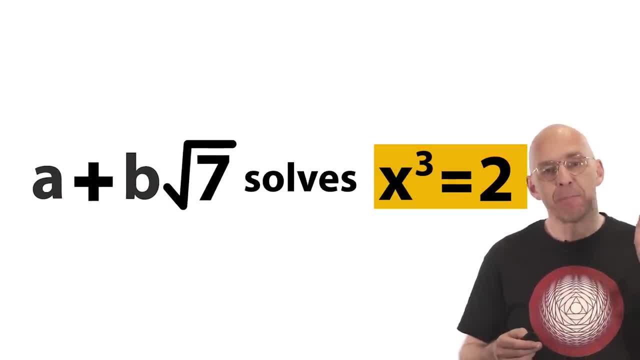 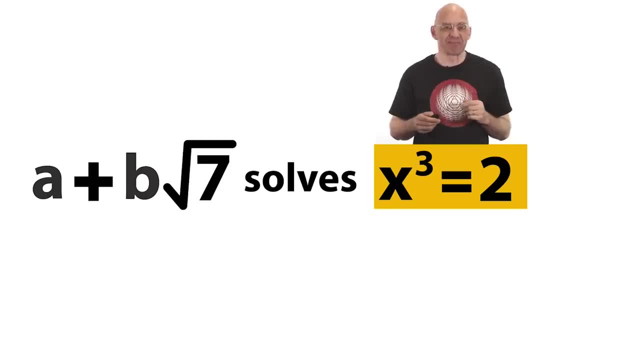 is a. If a plus b root 7 solves this equation, then a minus b root 7 does so too. Ok, you ready, Then here we go. So, when in doubt calculate, So moving the 2 to the left, plugging our root 70 thing in and carefully expanding. 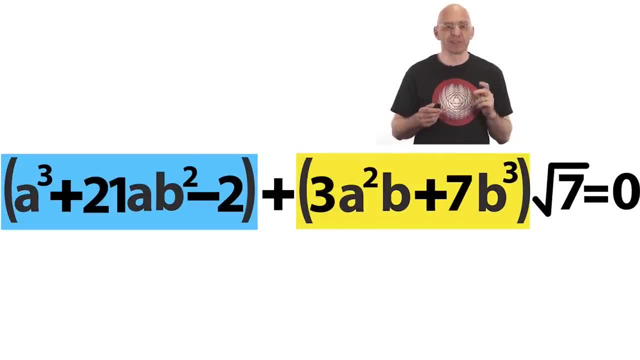 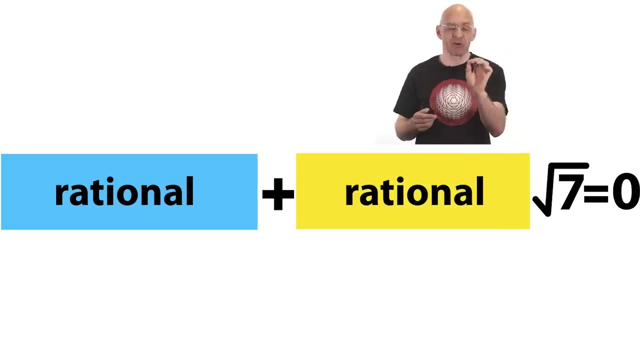 we get. let's see all of this mess. ok, But since we assumed a and b are rational numbers, the blue and the yellow numbers must be rational. But then, much more than being rational, the yellow number must be exactly zero. Why? Because? 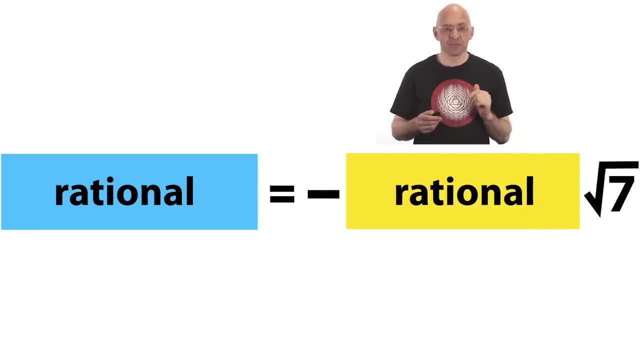 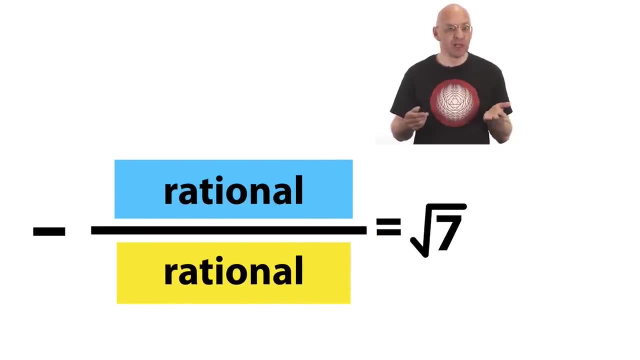 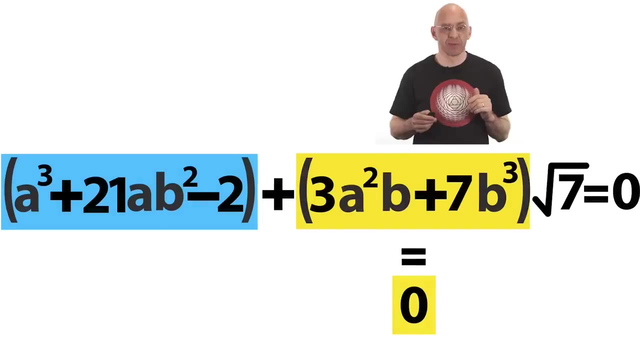 if it weren't, we could solve for root 7 like this, And that would mean root 7 is a quotient of rational numbers and so would also be rational. We already know that this is not the case, So the yellow number is definitely equal to zero. 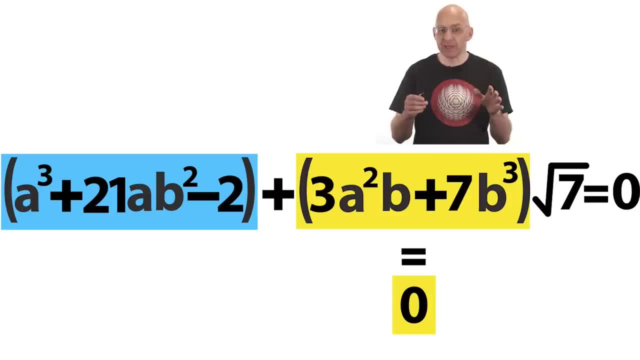 But with the whole left side being equal to zero, that means that the blue number has to be equal to zero too. And now everything is clear, right? Well, maybe not, But we're basically done. The key observation is that the blue expression only contains an even power of the number b and 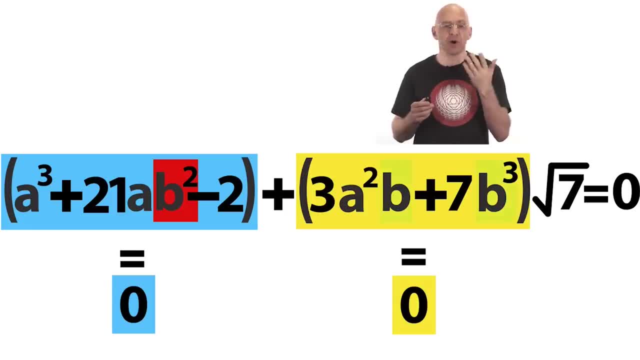 both terms in the yellow part have b to an odd power. So what? Here's the trick. Let's replace b with minus b. What changes? Well, the blue number is left unchanged, since the one minus sign gets squared away And because of the odd powers, the yellow becomes negative, like this. So there, the 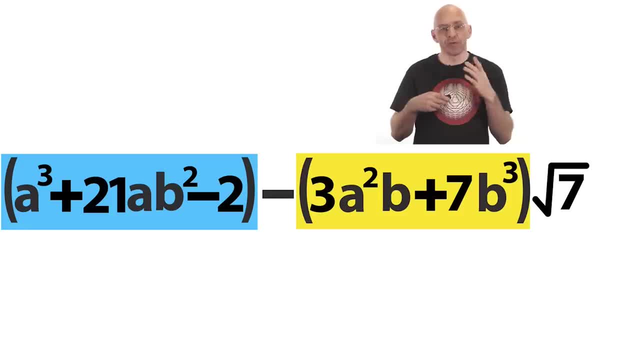 minus just goes out. That's it. So the overall effect of replacing b by minus b in this left side of our equation was simply to turn the plus sign in the middle into a minus. Overall, that's the only change, right. But since both blue and yellow are zero, the overall expression with the minus is still. 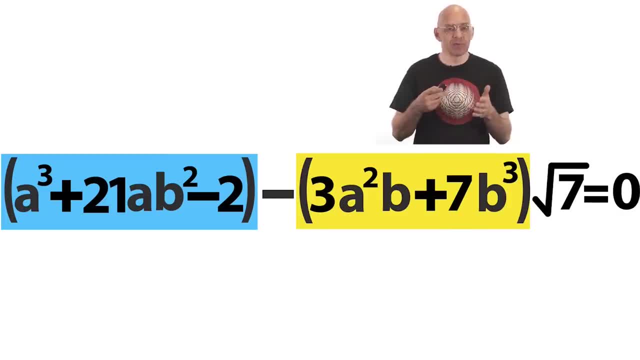 equal to zero. How does that help? Well, remember, the original blue and yellow expression was obtained by plugging our original root seventy number into x cubed minus two. But that means we get the new blue and yellow expression by replacing b in our number by 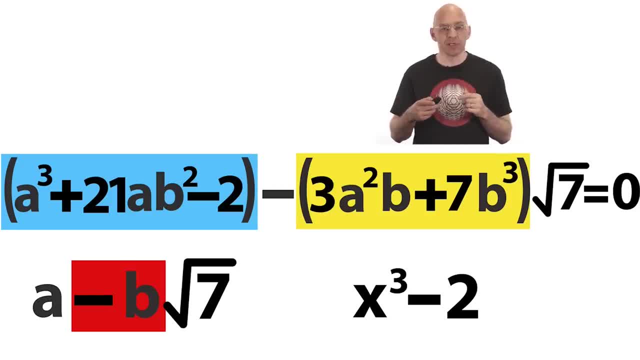 minus b And then again plugging this new number into x cubed minus two. But since the new blue and yellow expression is also equal to zero, this means that our new number is also a solution of our cubic equation Ta-da. 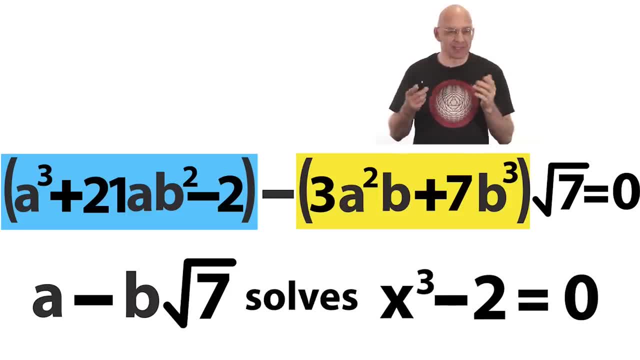 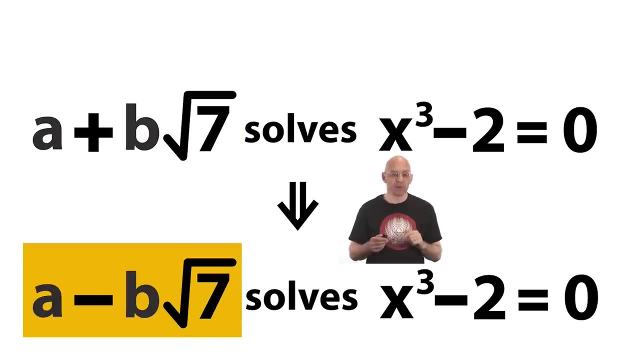 Well, maybe we have to go through this stuff again, but that's basically it right? Once again, the assumption that our original number a plus b root seven solves x cubed minus two is equal to zero. That implies that its conjugate, a minus b root seven, solves this equation as well. 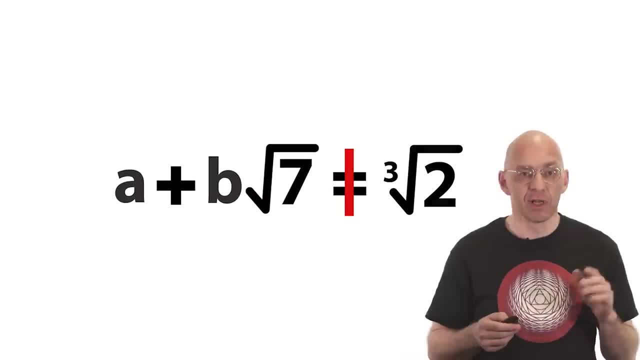 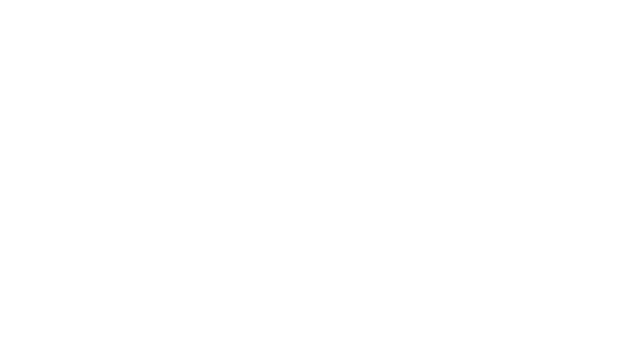 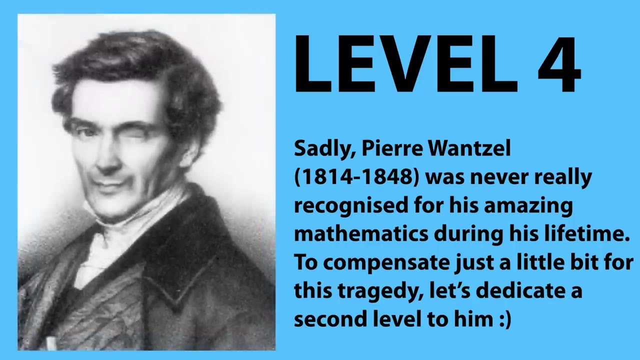 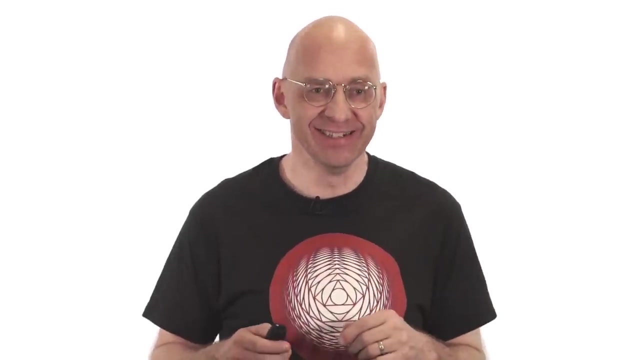 And this then implies the contradiction and we conclude that cube root of two cannot possibly be of the form a plus b root seven. Great, So you're still here. Thank you for watching. Bye, Bye, Fantastic. Now I promised you a big plot revelation. 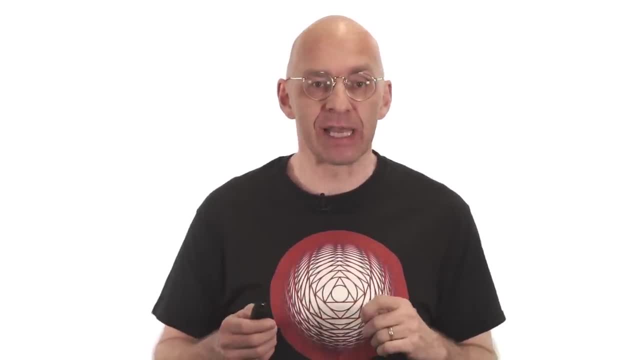 We're getting there. It turns out that we can iterate our a plus b root seven, proof by contradiction to conclude that the cube root of two is not equal to any square rooty number. To make the iteration work, we need to isolate the essential ingredients of our proof. 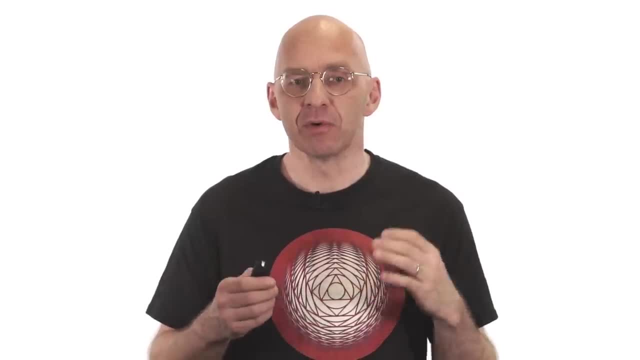 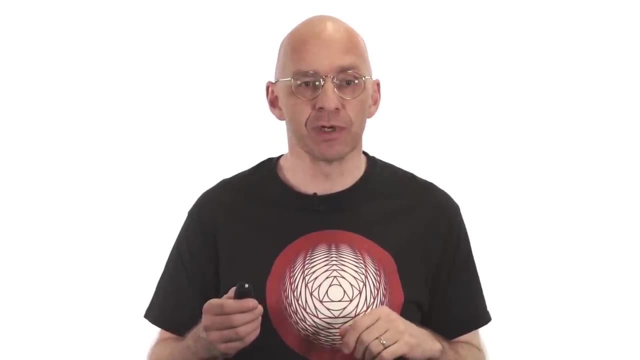 Turns out that these ingredients all have to do with the rational numbers which served as the foundation for what we're doing. There are four ingredients. First, we note that cube root of two is an irrational number. Second, we needed the property that adding, subtracting, multiplying and dividing of 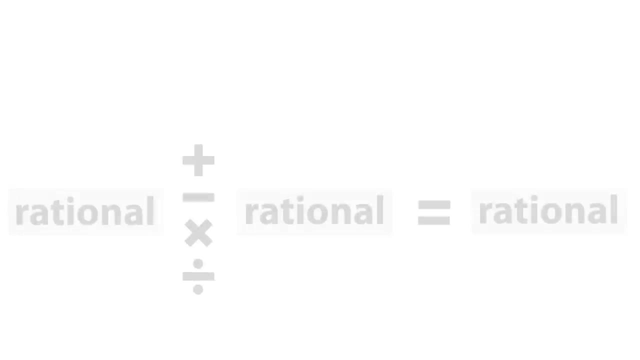 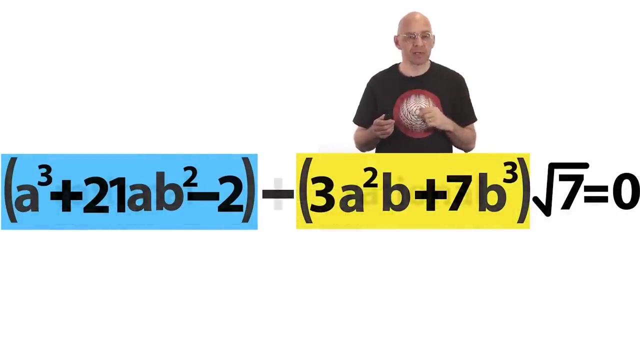 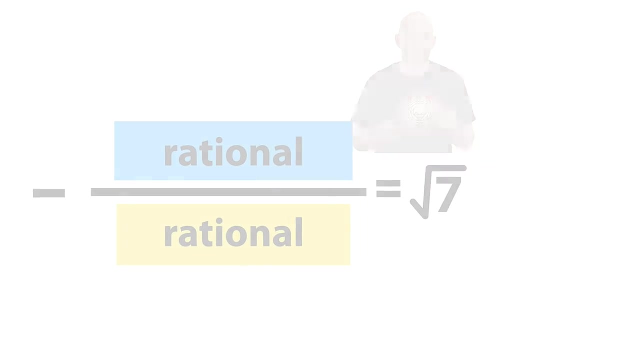 rational numbers always gives rational numbers. We needed this to be able to conclude that the blue and yellow numbers, being made up of rational numbers, are rational themselves. We also needed this ingredient when we argued that the ratio of two rational numbers is rational. The second ingredient: 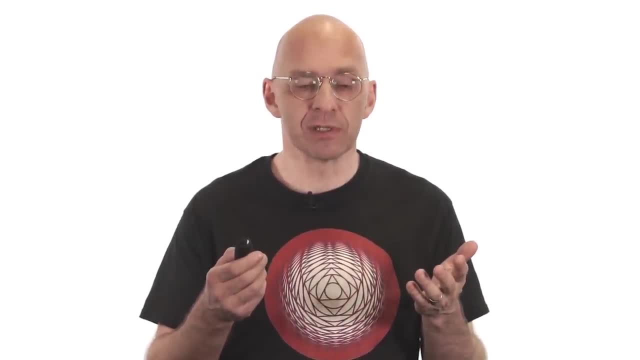 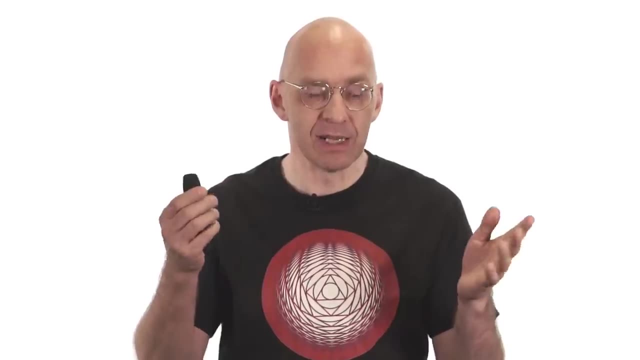 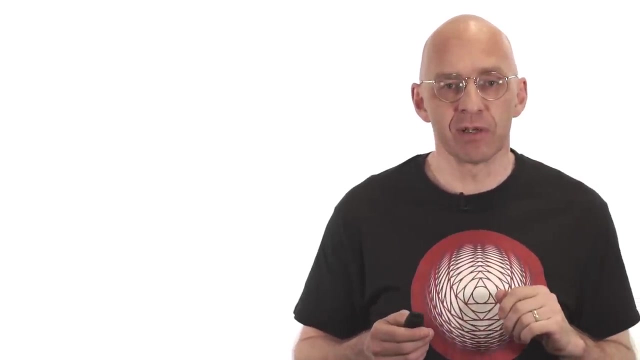 The property of being closed under the four arithmetic operations is described by saying that the set of rational numbers is a subfield of the field of all real numbers. It tells us that the rationals form a self-contained universe of numbers. Okay, The third important ingredient was the fact that seven inside the square root is a rational. 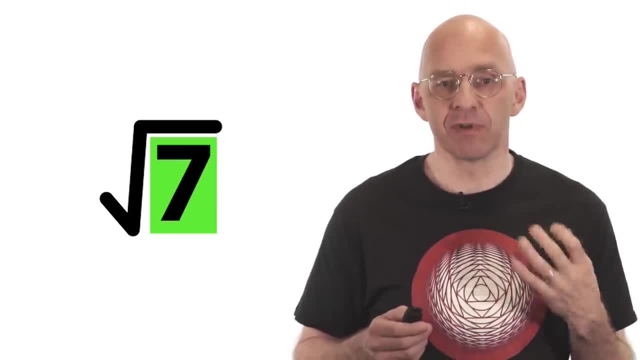 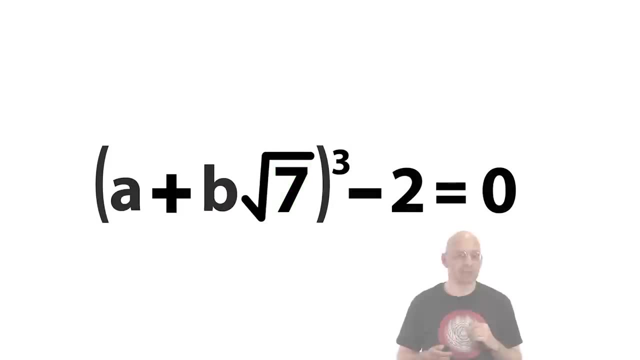 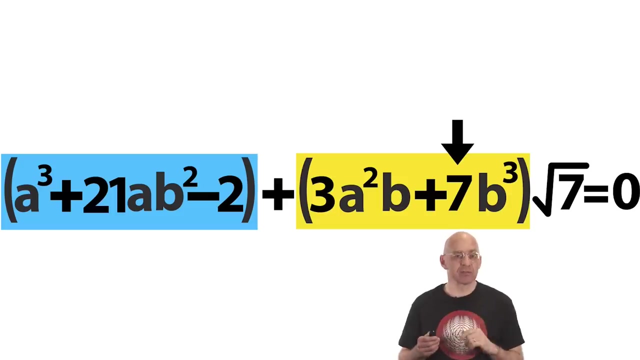 number Right. We needed seven to be rational because at various spots we used that square in the square root brought us back to a rational number. For example, when we expand it right at the beginning, that seven, there is the result of squaring the square root and we need that to be rational. 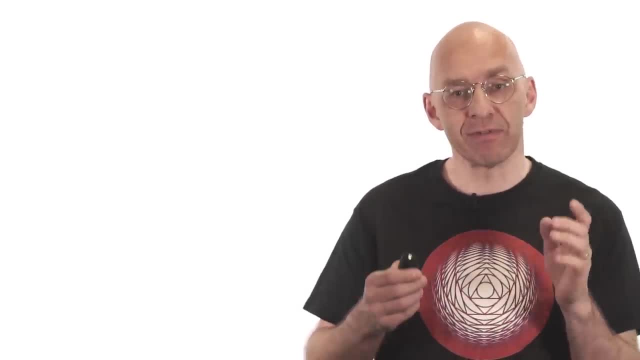 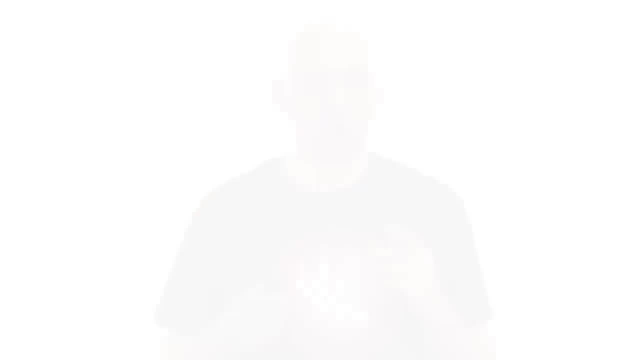 The last ingredient of our proof was the fact that, although seven is a rational number, its square root is not. We used this in two spots. Okay, To summarize, our magic ingredients are: The cube root of two is not irrational, It is a rational number. 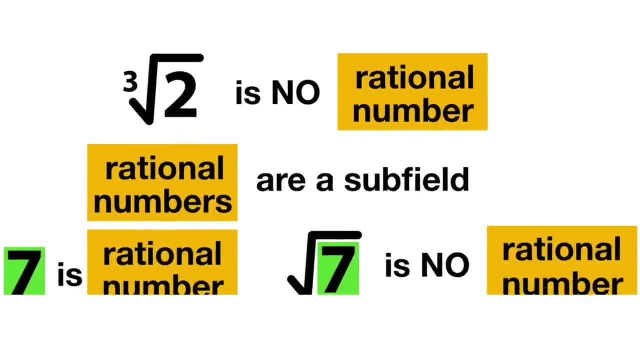 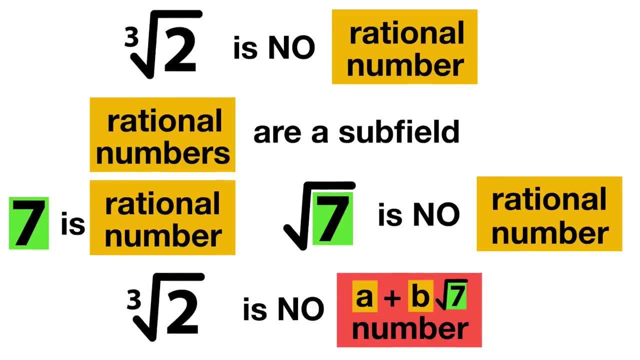 Rational numbers form a subfield. Seven is rational, Square root of seven is not, And from all that follows that cube root of two is not one of the red numbers. Okay, Now it turns out that the red numbers themselves are also a subfield. 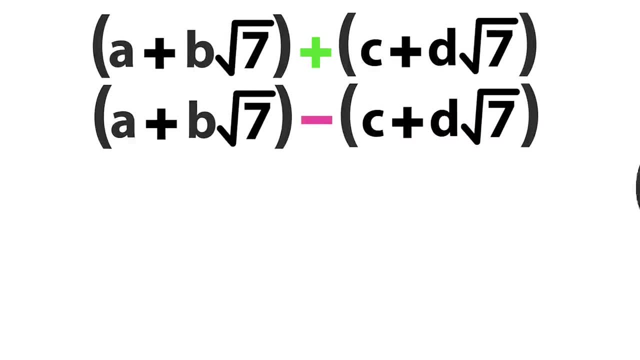 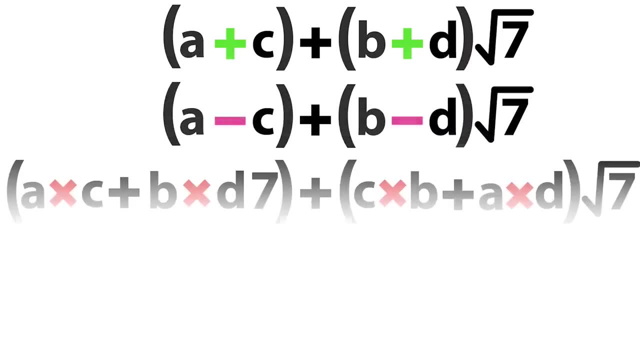 That is, if you add, subtract, multiply or divide. If you divide two root seven in numbers, then you again get a root seven in number. They are like this, All straightforward, except for the division, which involves a conjugate trick that some 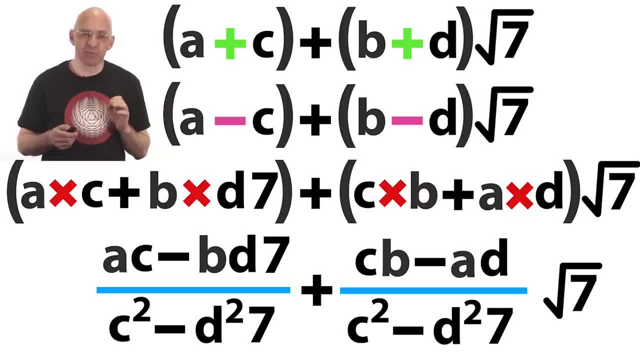 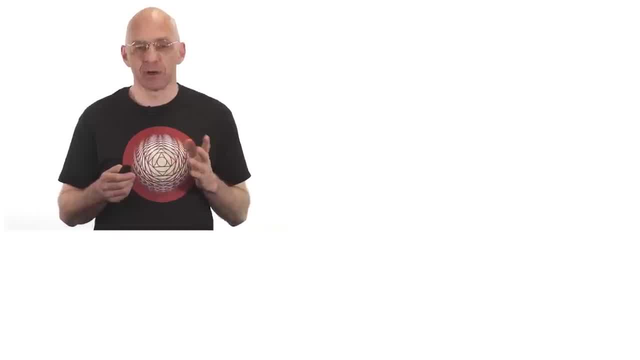 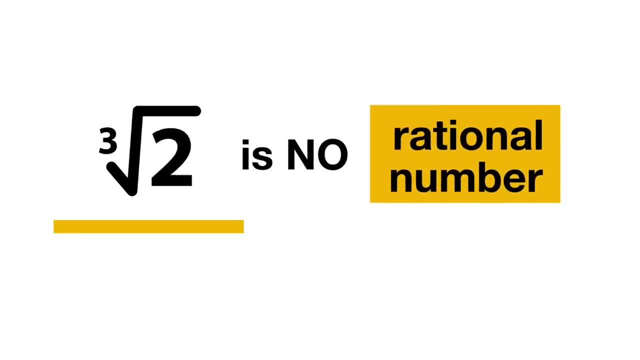 of you may remember from school And you can worry about division by zero if you are the worrying type. Challenge for you is to fill in the details in the comments. Okay, Ingredients again. Cube root of two is not a rational number. Rational numbers are a subfield. 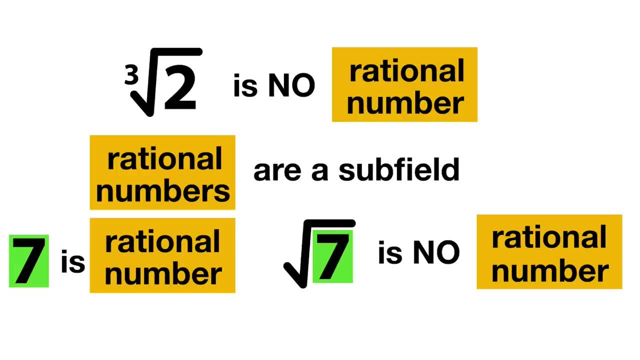 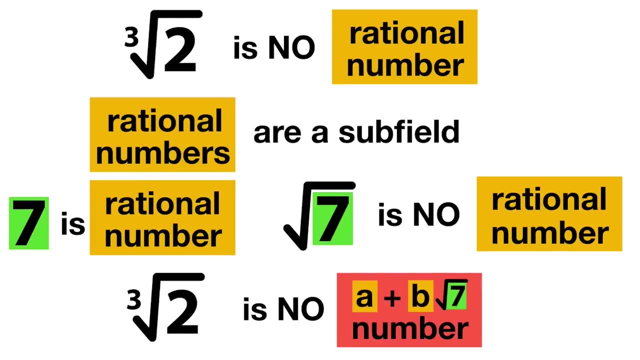 Seven is rational, Square root of seven is not. From this it follows that cube root of two is not one of the red numbers. Now the red numbers themselves are a subfield, And now things are supposed to repeat. So what comes next? 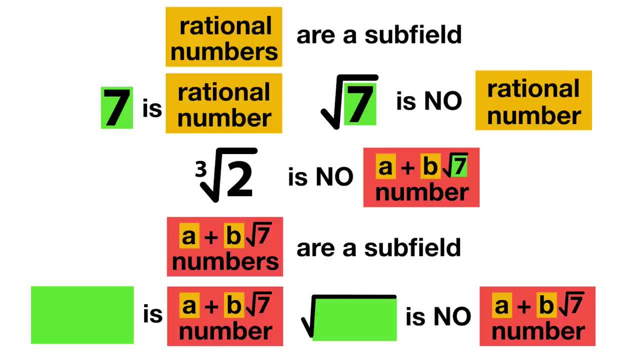 Well, something like this. So what we need is a number that is red but whose square root is not Okay, And I'll just give you one Okay. So one plus root seven is such a number, And root one plus root seven is not a red number. 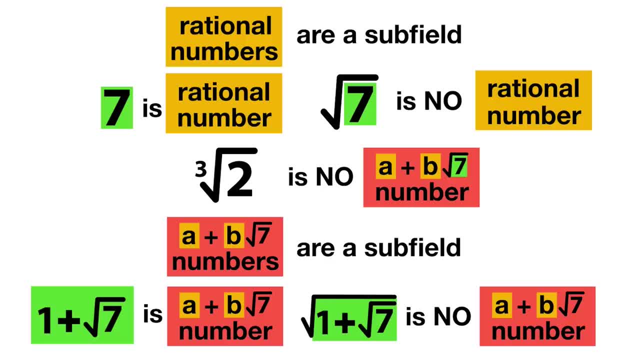 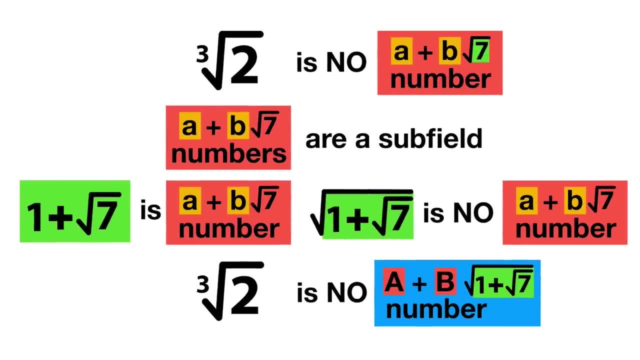 And now, with exactly the same arguments as before, we can conclude that all these blue numbers are not candidates for anything that can be equal to cube root two. And now things repeat again, because the blue numbers can also be seen to be a subfield, With exactly the same arguments as before. 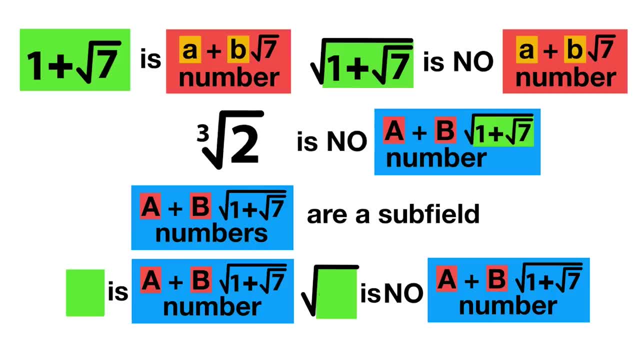 And now, well, repeat, So we need a line here, So we need a number that is blue but whose square root is not, And there's lots and lots of possibilities. So I'll just give you one again. Eighty-six divided by five is such a number. 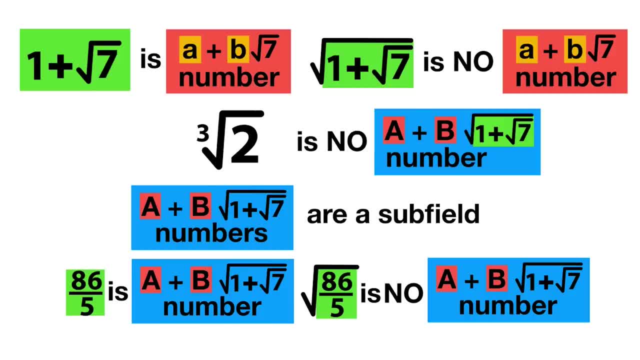 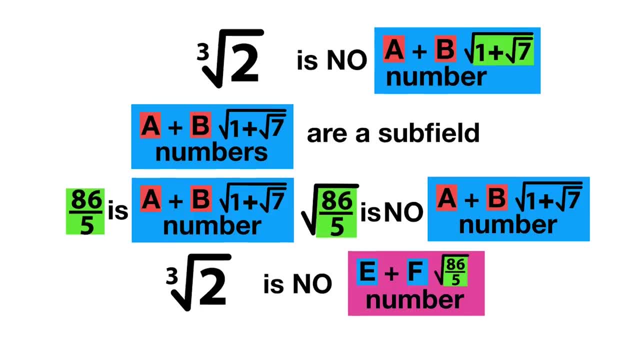 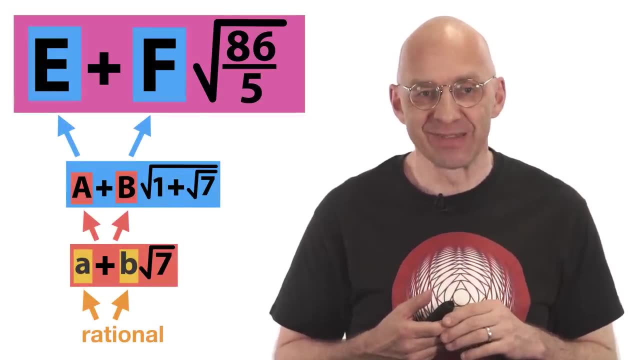 And now with exactly the same arguments as before. it follows that cube root of two is not one of the pink numbers, And we can go on like this. At this stage, perhaps you're feeling a little rooted. as we say in Australia: Time to catch our breath and take stock. 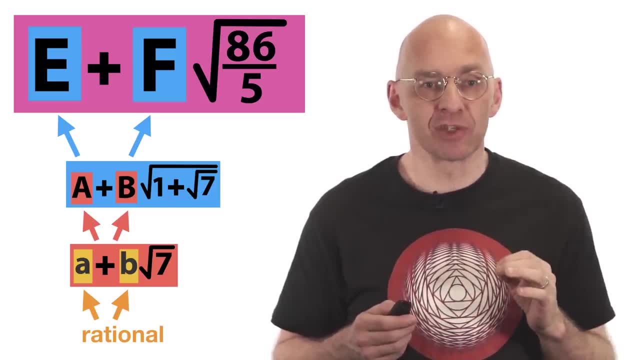 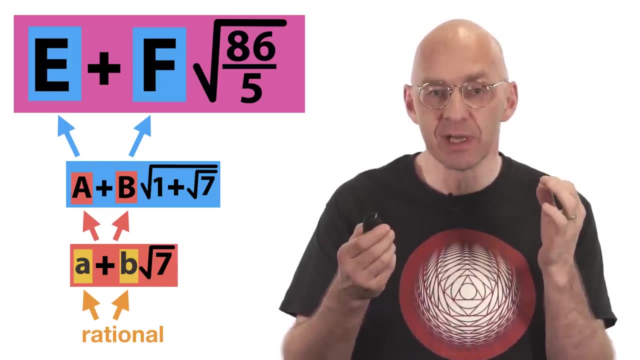 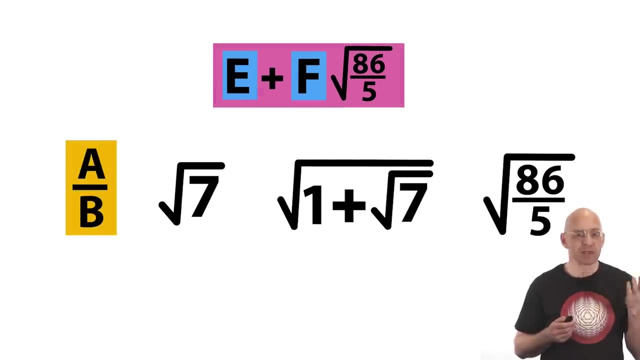 The field property of the subworlds of numbers that we've been looking at shows that the final pink numbers are exactly the numbers that can be constructed by combining the rational numbers and these three rooty expressions with the usual arithmetic: Adding, subtracting, multiplying and dividing. 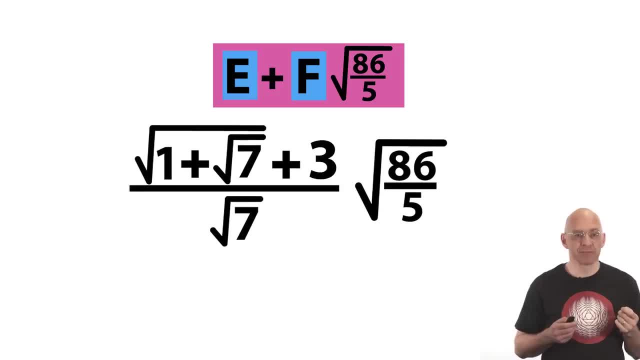 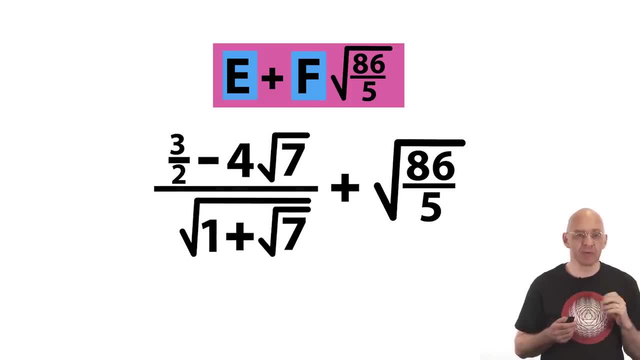 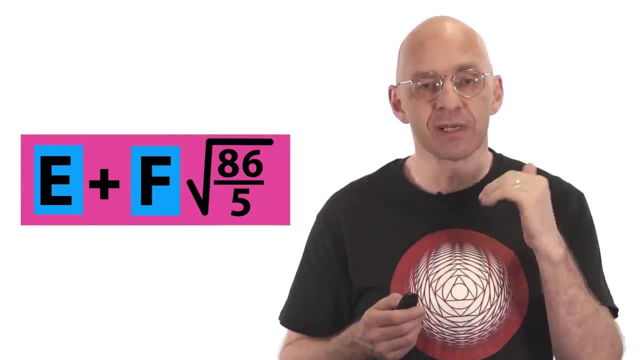 For example, this complicated rooty number is one of the pink numbers, Same here, Same for this one And this one, And because they are all pink numbers, none of them can equal cube root of two. Of course, any individual pink number can be ruled out using a calculator. 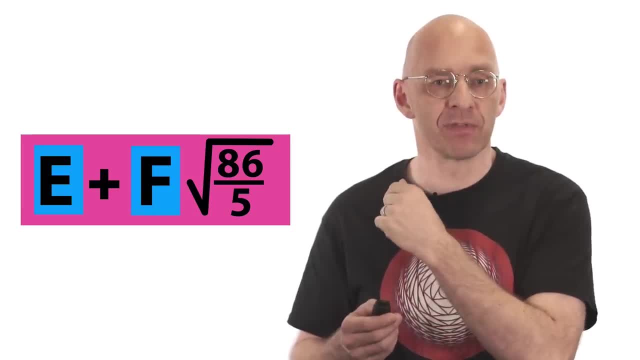 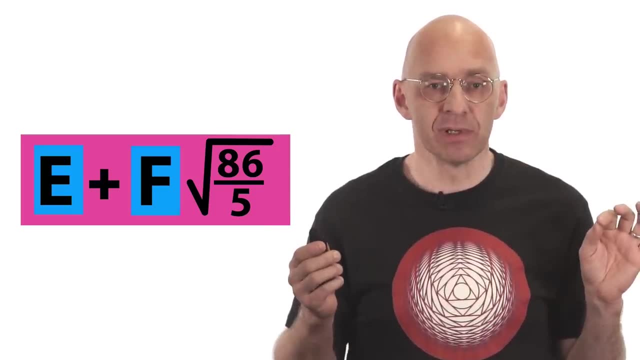 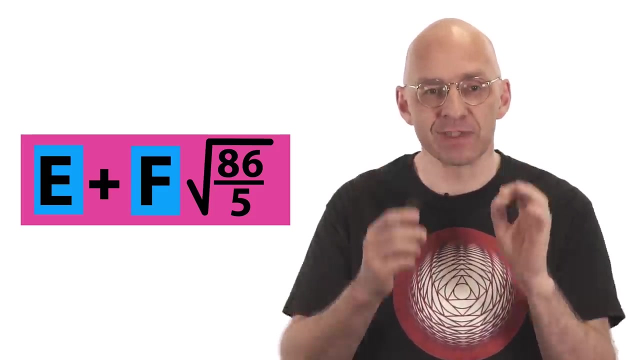 But the point is that we've ruled out all the pink numbers of that subfield And we can go to bigger and bigger subfields. Given any square rooty number, we can start from the rational numbers and, by iterating the extension process In a finite number of steps, a subfield that contains that particular square rooty number. 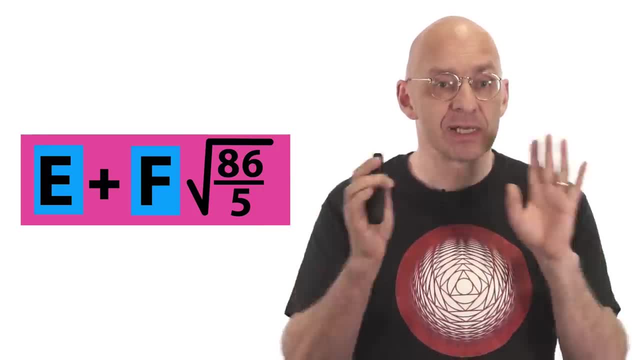 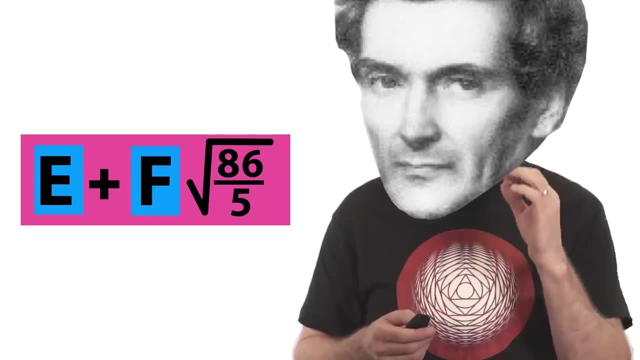 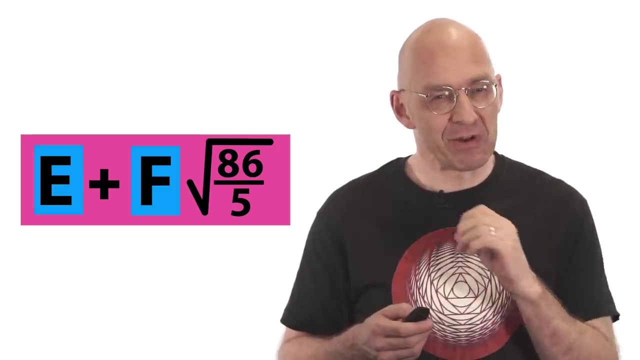 And so that square rooty number, any square rooty number, cannot be cube root of two. And that's it That completes the proof that cube root of two is not a square rooty number and therefore that the cube cannot be doubled with ruler and compass. 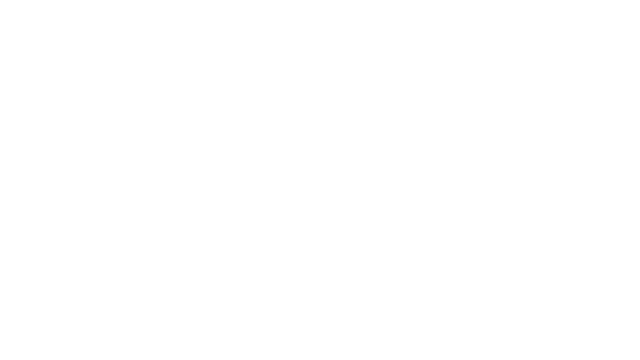 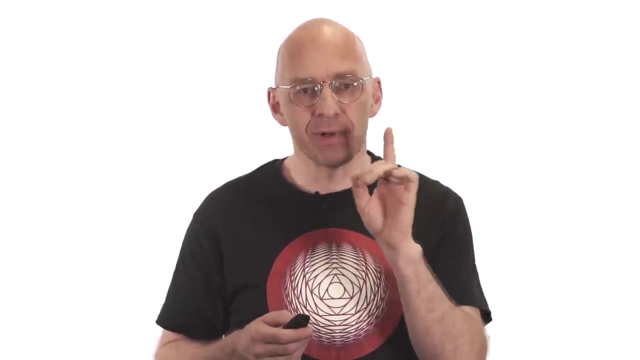 Very hard work, but also very, very nice, Don't you think So? before going to the next level, there's just a little tidying up to do. Remember that we knew, or we assumed, or you simply trusted me, that root, one plus root. 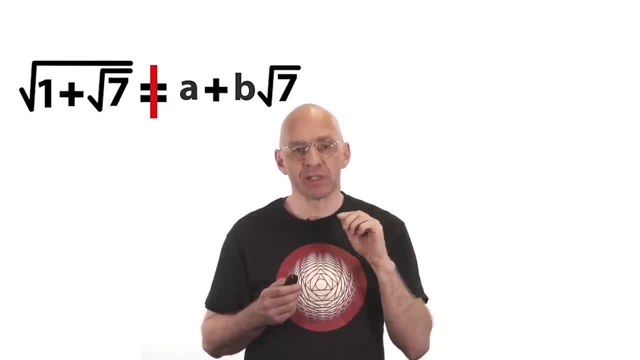 seven is not part of the a plus b root seven subfield, And that root eighty six divided by five is not part of the last subfield, And so on. But even if root one plus root seven was part of the last subfield, root one plus root seven. 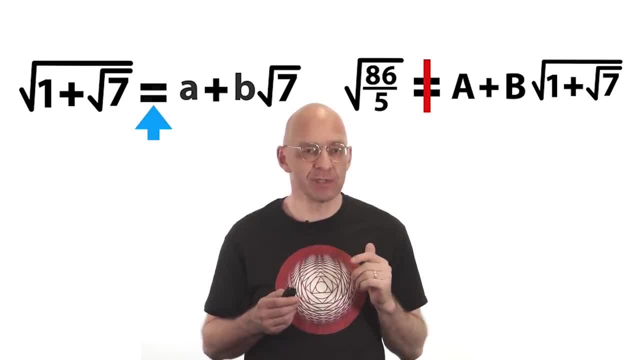 is not part of the last subfield And so on. But even if root one plus root seven is not part of the last subfield, root one plus root seven is not part of the last subfield. That would just mean that to get to this point, we would need one less step of the extension. 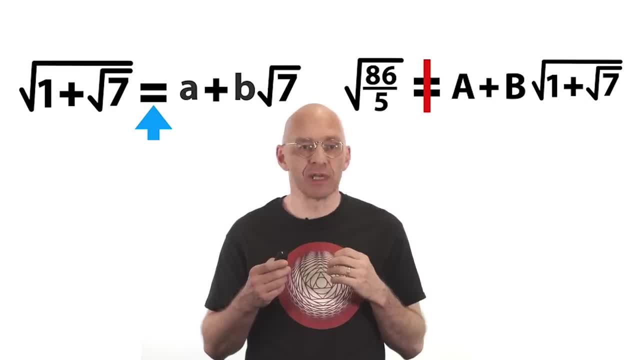 process. It's the same for all the square roots that go into building our subfield extensions. If the subfield is enlarged, we know how to handle it. if not, then nothing has changed. All that matters is that whenever our subfield is, 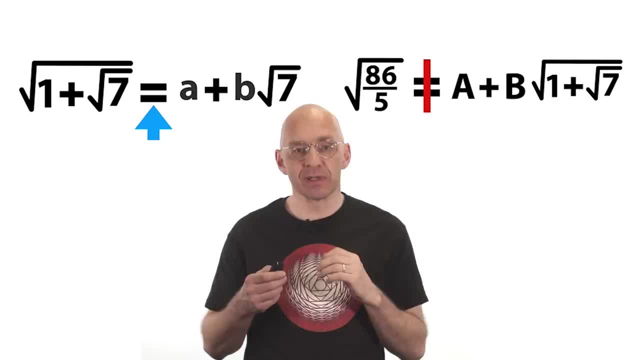 enlarged, we are guaranteed that the new subfield still cannot contain cube root of 2.. And this really finishes the proof that no square root in number is equal to cube root of 2.. In turn, this shows that it is impossible to double a cube. 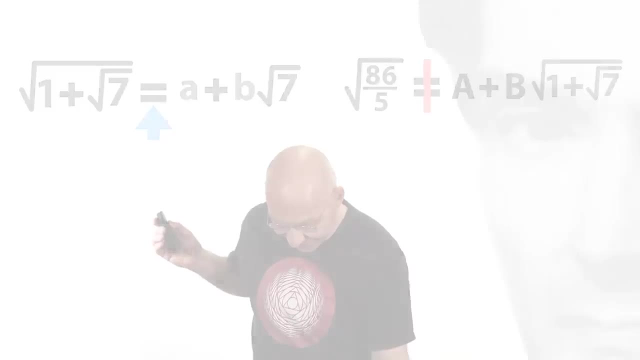 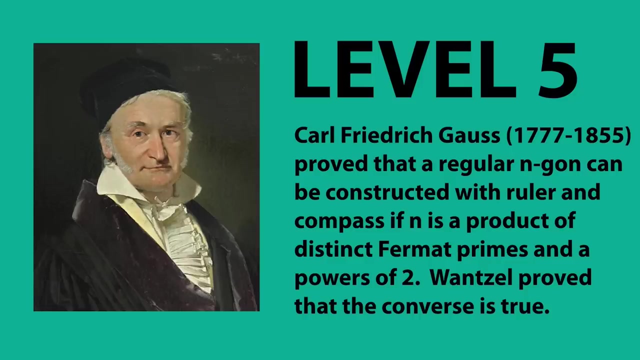 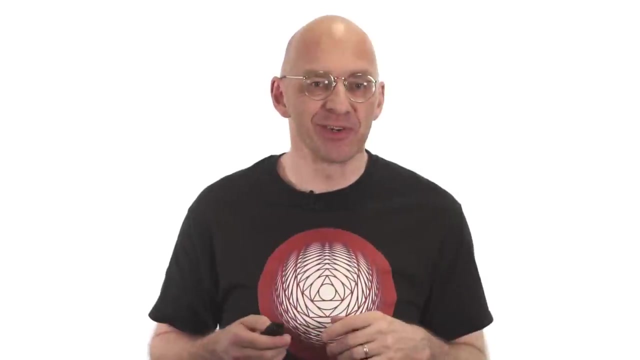 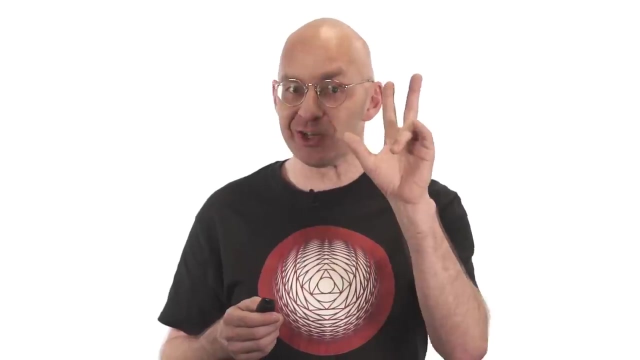 just using ruler and compass. What an ingenious argument, don't you think? But there were four problems that I promised to solve in this video: One down after quite a fight and still three to go. How long a video is this going to be? Well, not that much longer, It turns out. 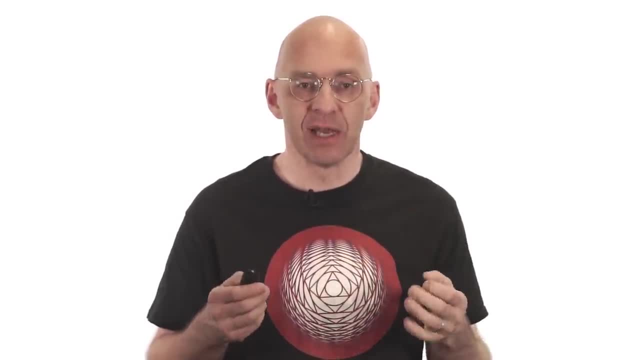 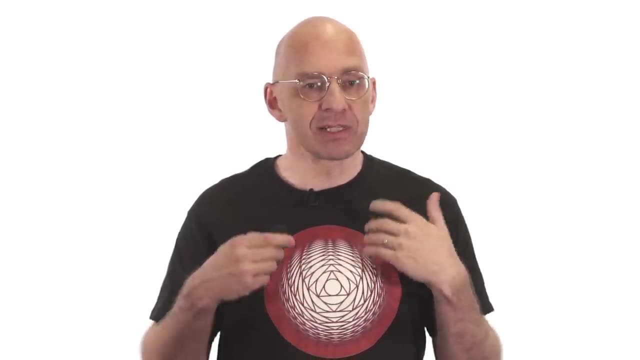 that proving the impossibility of trisecting angles and constructing a regular heptagon with ruler and compass can be taken care of in a very similar fashion, Just like doubling the cube boiled down to showing that the solution of the cubic equation x cubed minus 2, is 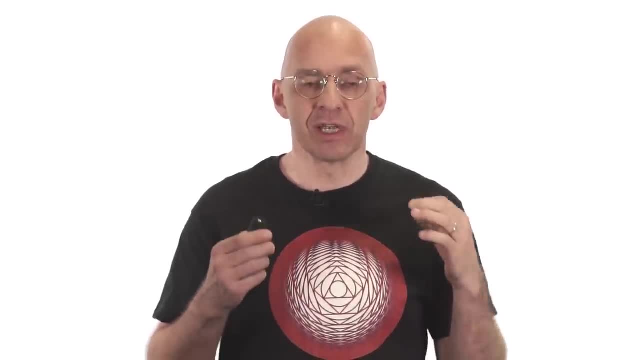 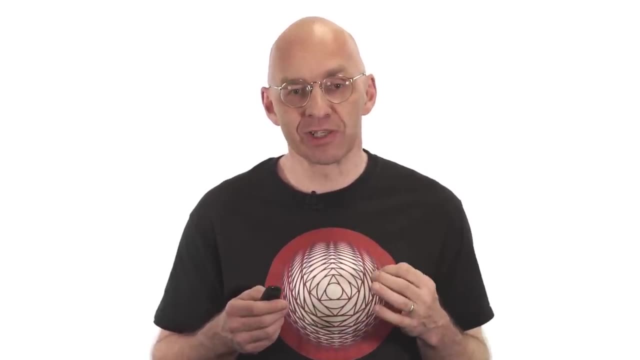 equal to 0 cannot be a square root expression. showing the impossibility of trisecting and heptagoning reduces to showing that the roots of two other cubic equations cannot be square root expressions. First, trisecting an angle. 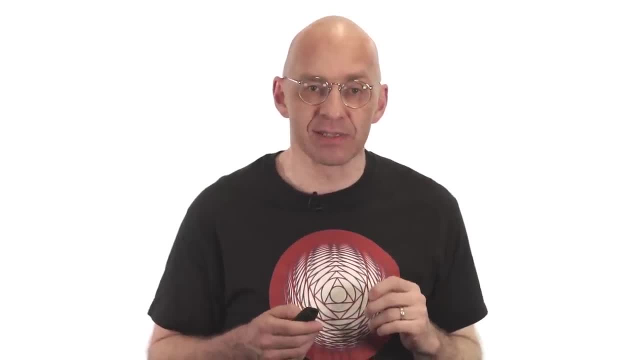 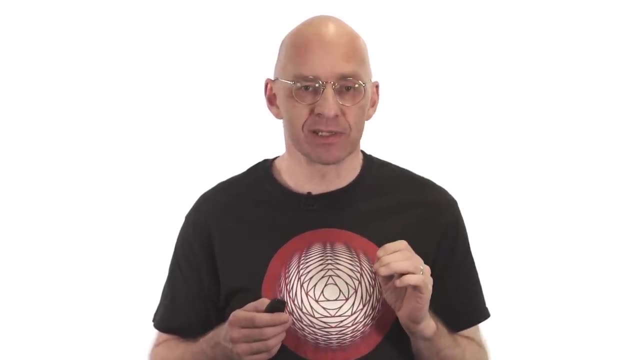 Of course some angles can be trisected. The angle 90 degrees, for example, is easy to trisect, But the point is that not all angles can be trisected, And to show this we just have to prove that one particular angle. 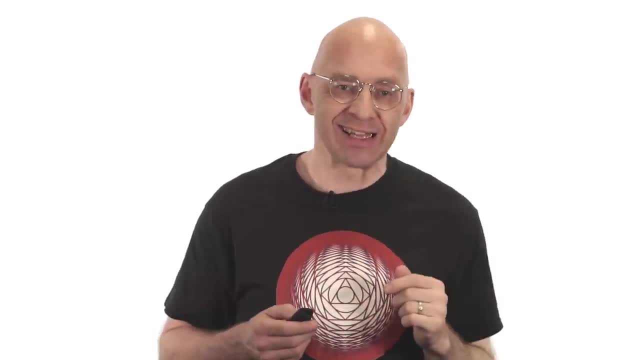 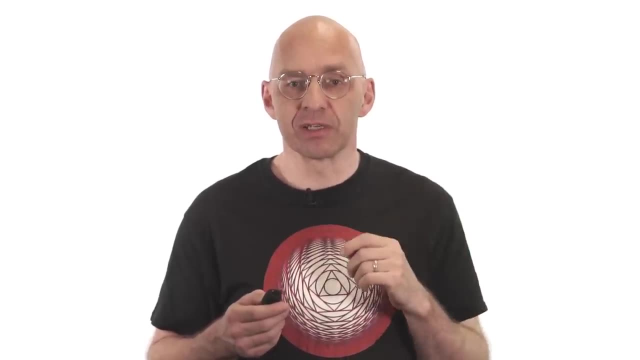 cannot be trisected, and we've chosen 60 degrees as our victim. Here's a quick run-through of how you show that ruler and compass cannot be used for constructing 20 degree angles. That then proves the impossibility of trisecting. 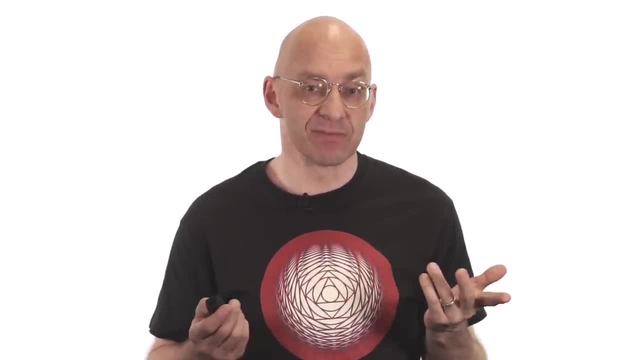 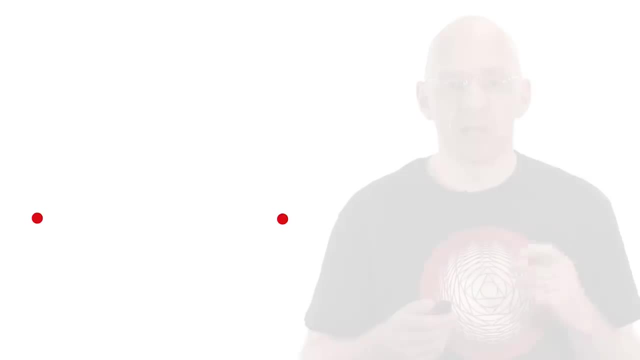 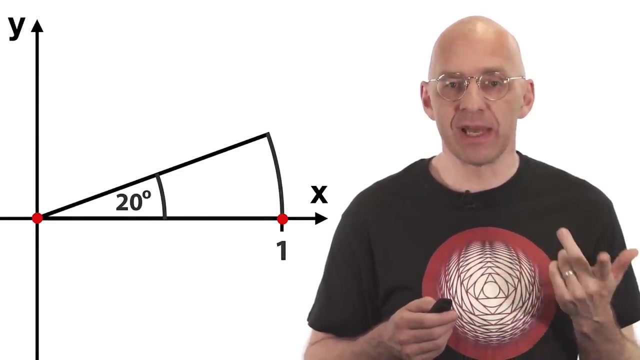 a constructible angle: 60 degrees. And you guessed it, it will be a proof by contradiction. So let's assume that, starting with our two points, it was possible to construct a 20 degree angle. Then we can transfer the angle to the origin like this, And then constructing this perpendicular also gives us the 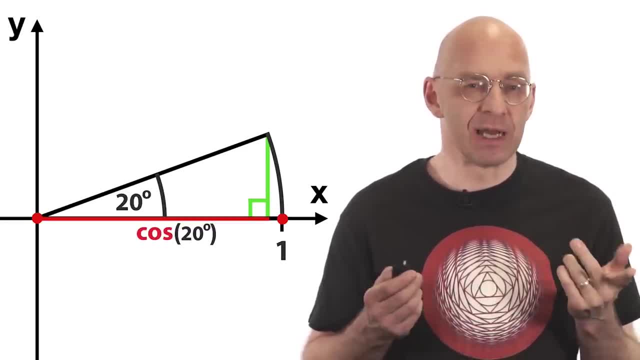 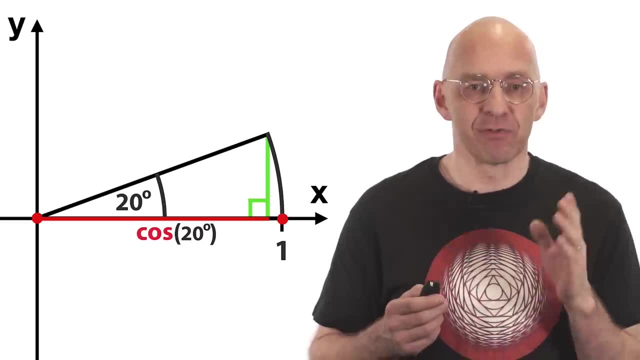 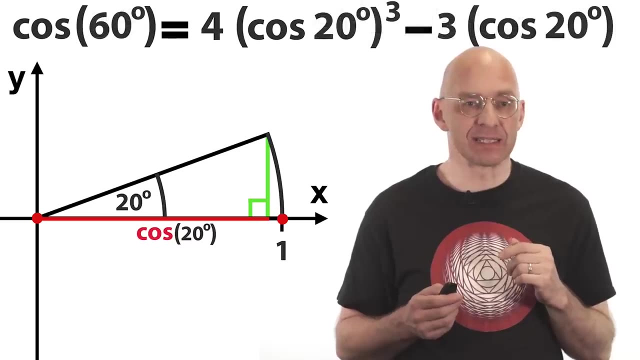 cosine of 20 degrees. Time to dust off your high school trick. Remember your double angle formulas? Well, there are also triple angle formulas, and the formula for the cosine is this: Substituting 20 degrees for theta, we get this. The cosine of 60 degrees is 1 half. 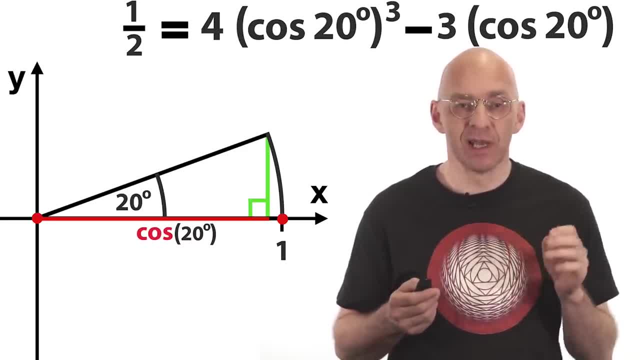 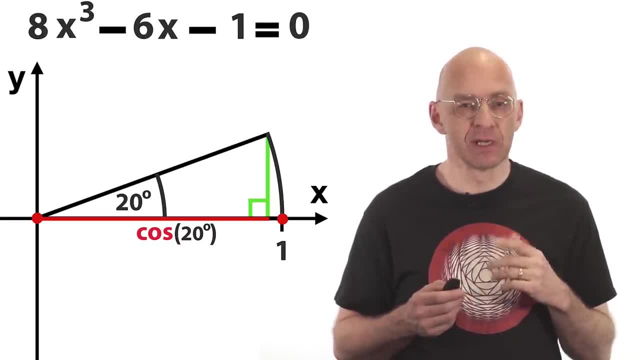 and this means that the cosine of 20 degrees is a solution of this cubic equation. here Now we can use the rational root theorem from two videos ago to prove in the blink of an eye that this equation has no rational roots. And because we are again dealing with a cubic equation, things proceed. 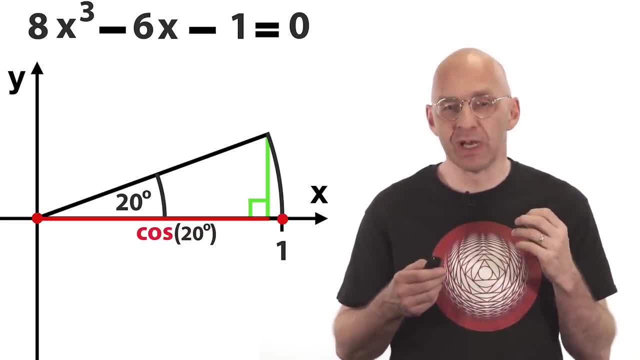 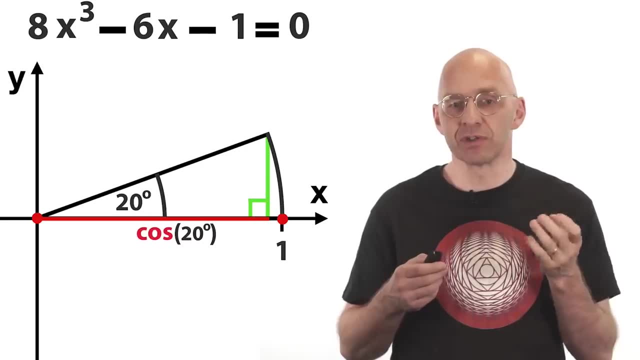 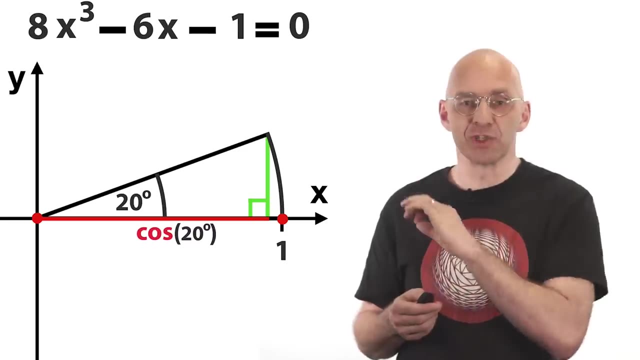 very much along the lines of the cube root of 2 proof. In particular, assuming that a solution of this equation is contained in a square rooty extension field forces the conclusion that there is also a solution in the smaller subfield. And this then gives the usual contradiction Challenge for you. Fill in. 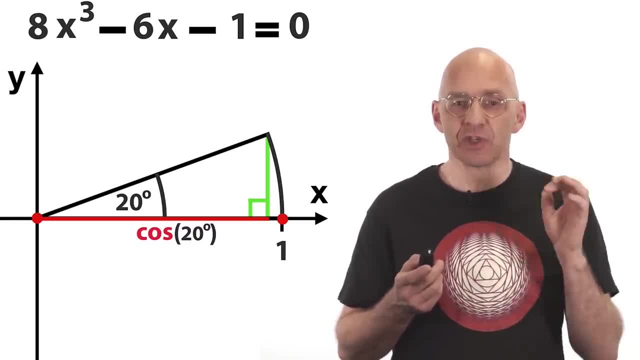 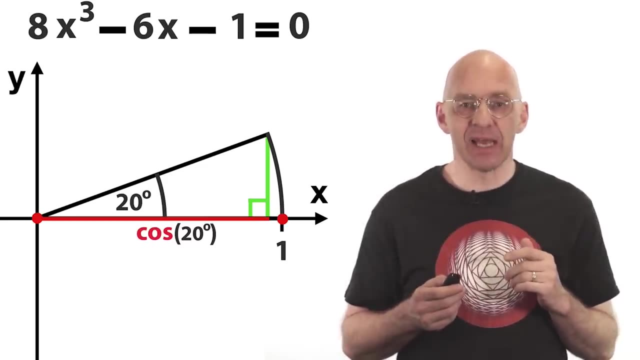 the details. One slight difference: you'll have to deal with The cubic, for the trisection has three real solutions rather than just one. For those who get lost or just play in exhaustion, I can understand. I'll also provide some links to the write-up And on to. 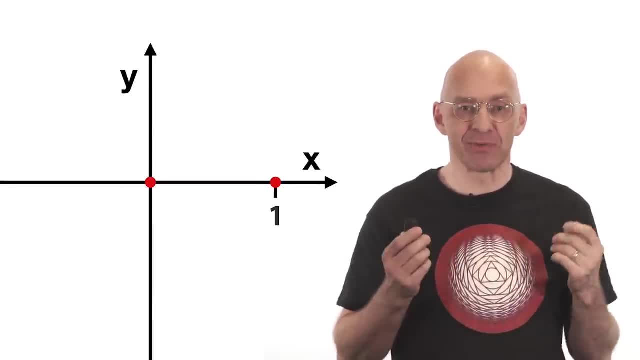 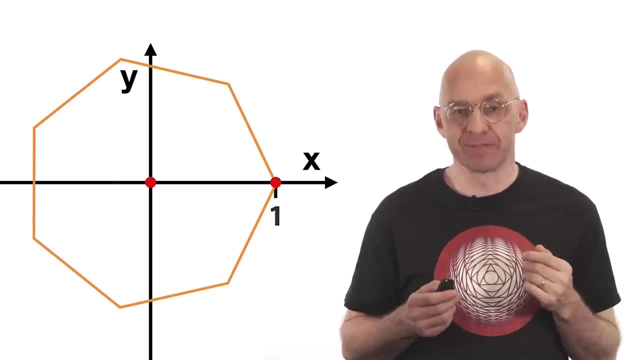 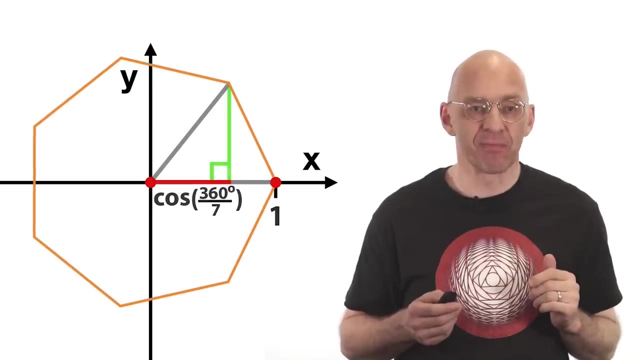 heptagons. If it was possible to construct a regular heptagon with a Wollein compass, then, starting with the usual two points, it'd be possible to transfer the heptagon here. This would mean that it was possible to construct a number cosine of 360, divided by 7 degrees. There, that creature, And then 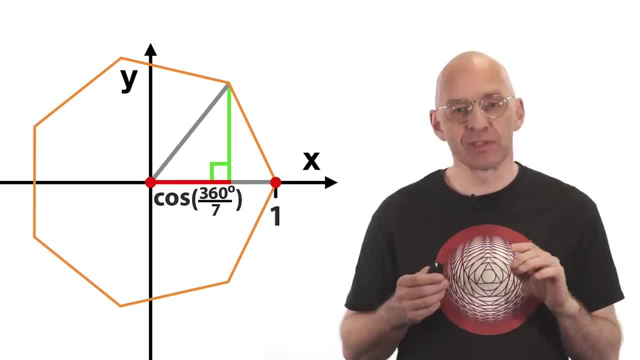 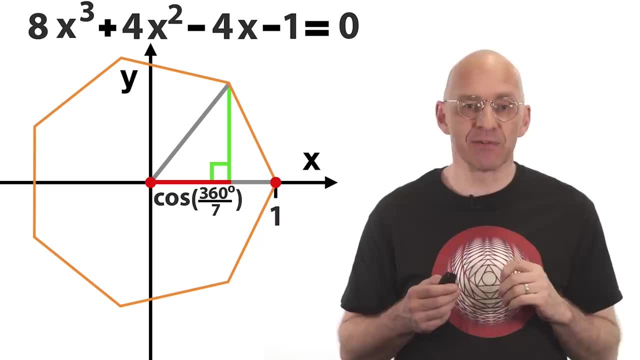 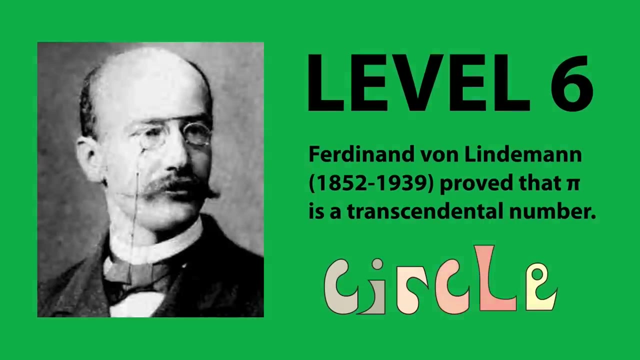 it's fiddly, but it can be shown that this cosine is a solution to this cubic equation there And it's straight sailing from there. Again, I'd say, first try to fill in the details yourself in the comments and if you get desperate, follow the links in the description. 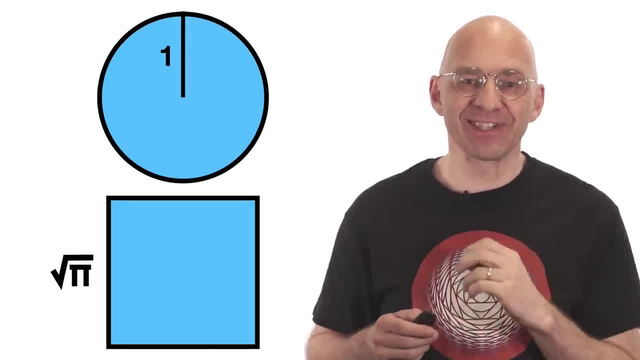 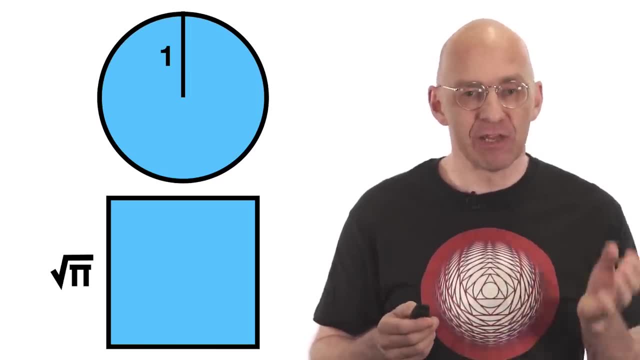 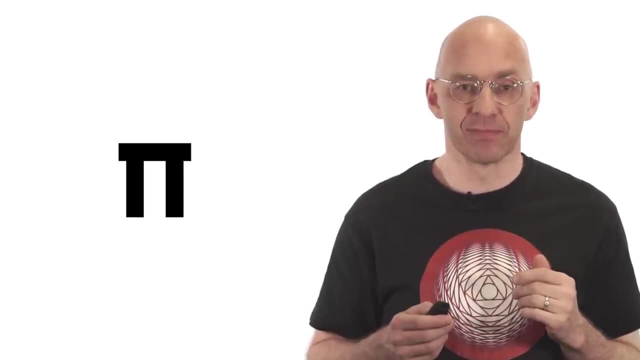 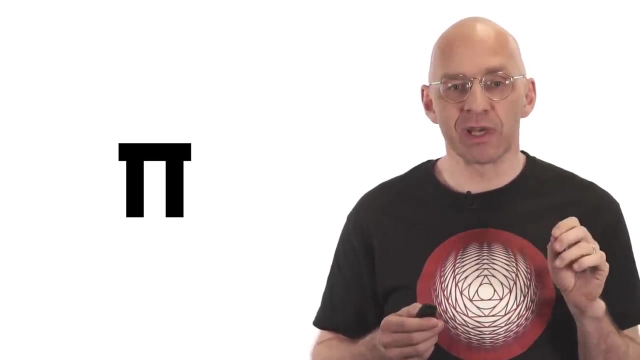 Finally, finally, finally, What about squaring the circle? And what about using Wollein compass to construct the number root pi? Well, if root pi was constructible, then its square, the number pi, would also be constructible. However, it turns out that all square rooty numbers are algebraic. That is all square. 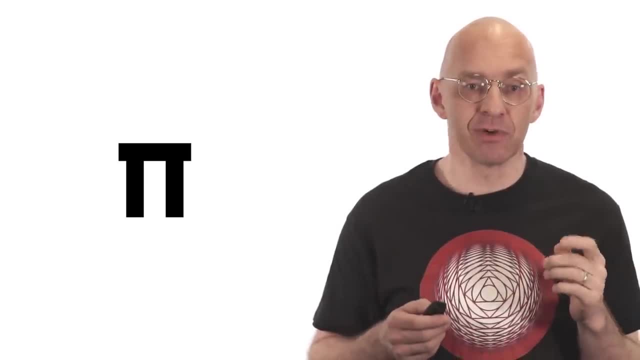 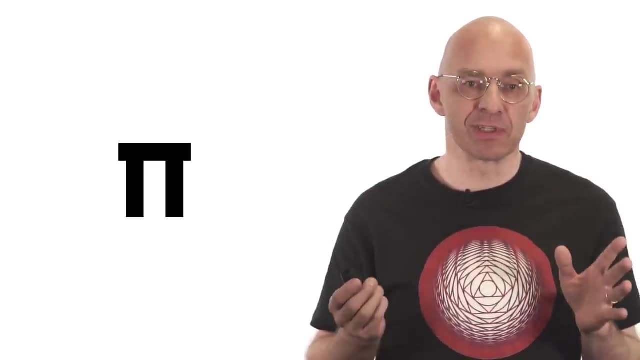 rooty numbers, and in fact all rooty numbers, are solutions of polynomial equations with integer coefficients. But pi is not. as we showed you in a previous masterclass Mathologer video, pi is a transcendental number. It is not the solution of such a. 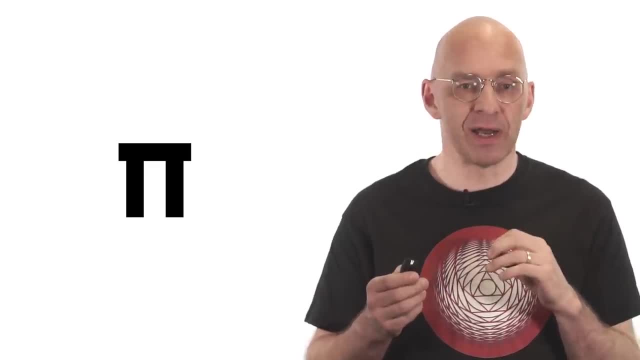 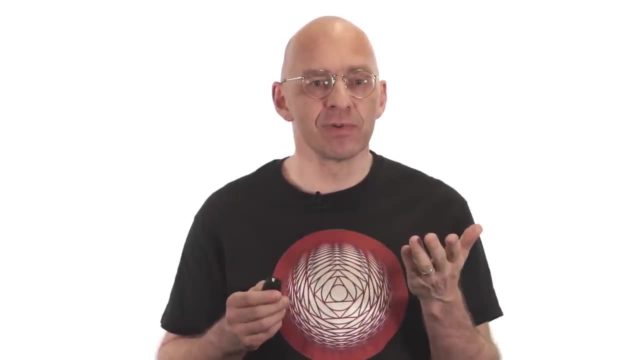 polynomial equation. This proves that pi cannot be constructed, and that's all there is to it. But to nail down the last little bit of the proof, how does one prove that all square rooty numbers are algebraic? It turns out to be pretty. 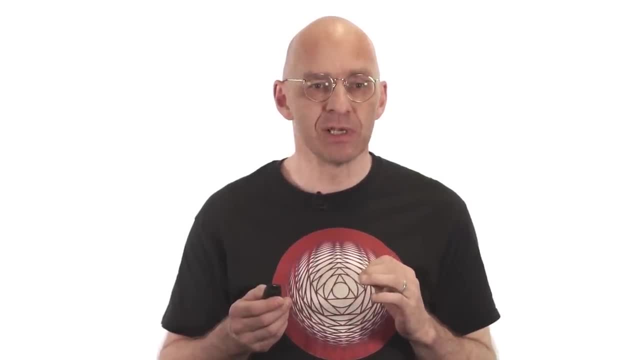 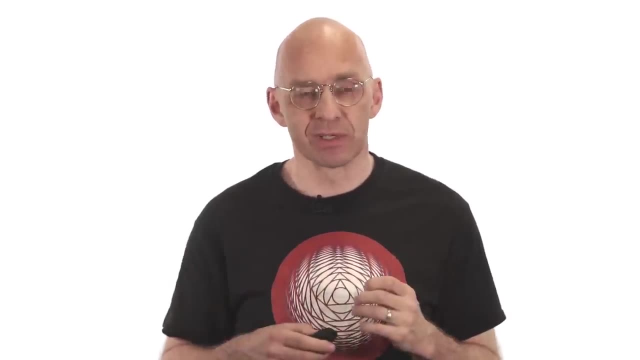 easy. The idea is to start with a square rooty expression, set it equal to x and then unravel the resulting equation, successively isolating and squaring away the square roots. Eventually, all that is left are integers and powers of x To. 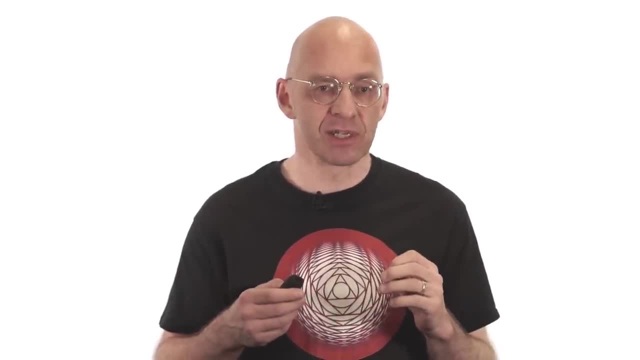 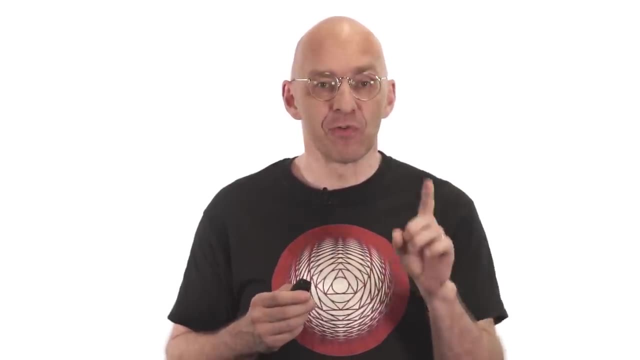 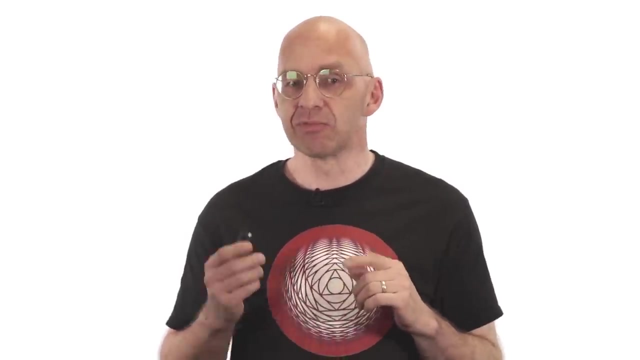 give you some intuition, I'll finish this video with an animation of constructing such an equation for one of our previous scary square rooty expressions. But before the pretty ending, first let me finish with a few thoughts on impossibilities. Today's video was a tricky tour through some difficult 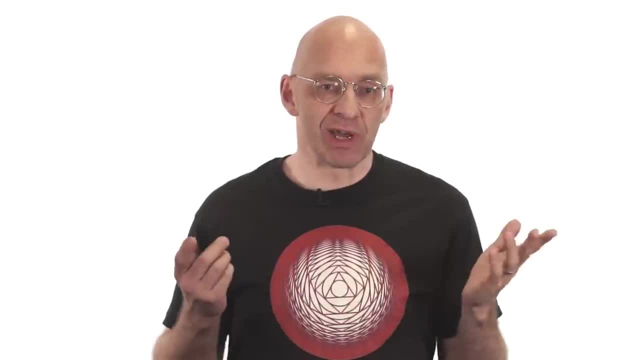 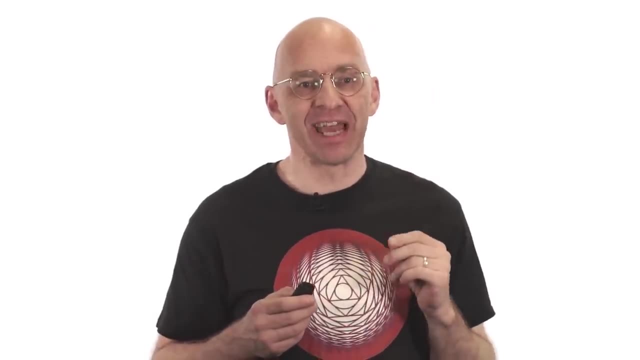 mathematics. It easily took me 200 hours to put it together And still, even after me and Marty there behind the camera have agonized and re-agonized over every detail of the video. it's tough going. I don't expect that everybody who watches 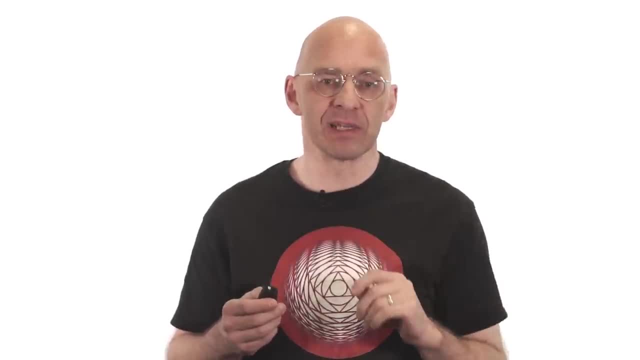 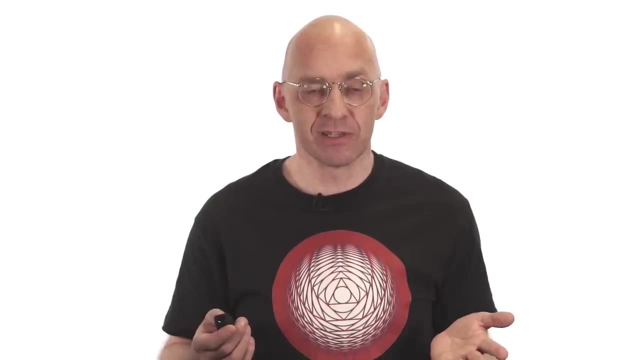 this will get everything in a first view. Don't feel bad if you don't Just give it another go and remember it took mathematicians a couple thousand years to sort out these ideas, and it took that long for a reason. And so if it takes you a few viewings and maybe a question or two in the 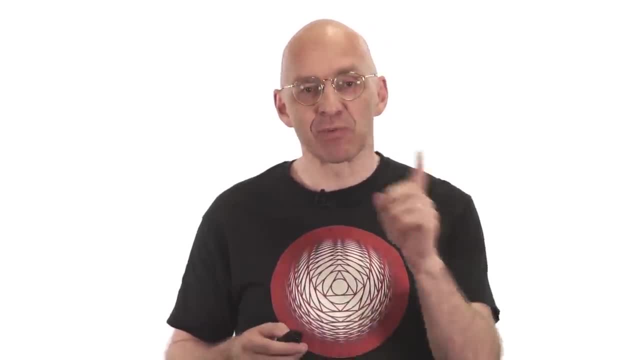 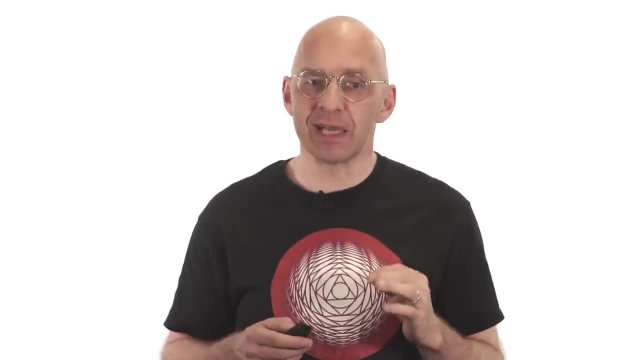 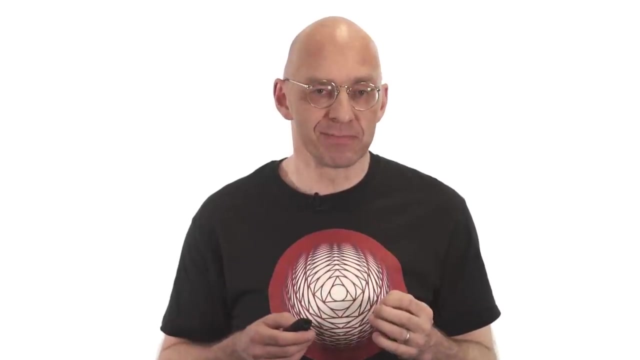 comments. that's perfectly fine, But there's one more thing. Every year I get at least a few people writing to me with the news that, after devoting anything from a few seconds to half a lifetime of study, they have managed to square a circle or have achieved some other impossibility. Of course, they're all. 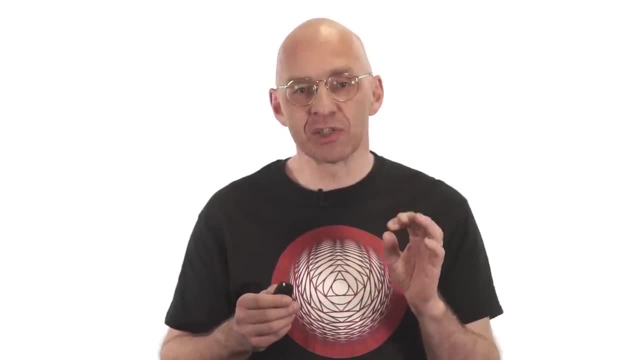 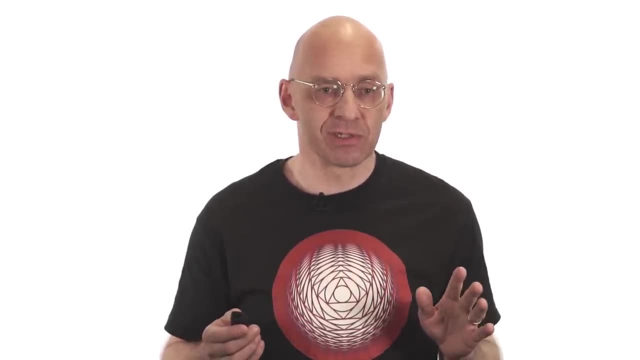 wrong. It's important to realize that if you change the rules of our game just a tiny, tiny little bit, it's then no problem at all to square the circle and so on, And this has been known since the days of Euclid. The plan is actually to 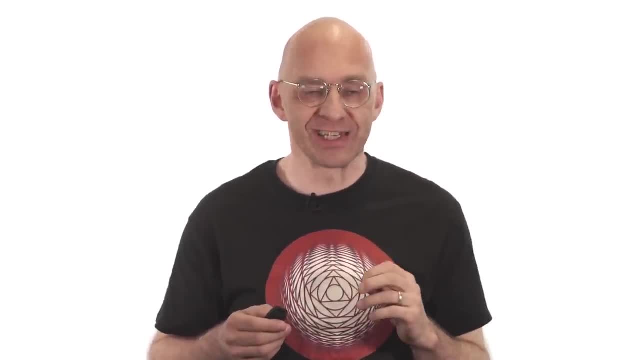 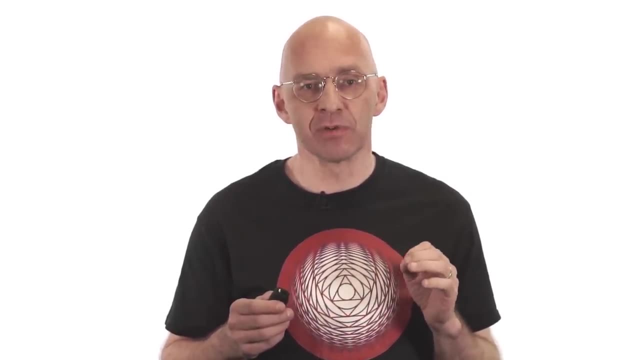 make another video about this fascinating topic of rule changing in the near future. Let's see. Anyway, it's very easy to misinterpret the rules of the Greek game and end up with false solutions of those ancient problems, Especially if you base your understanding on a bare-bones exposition. 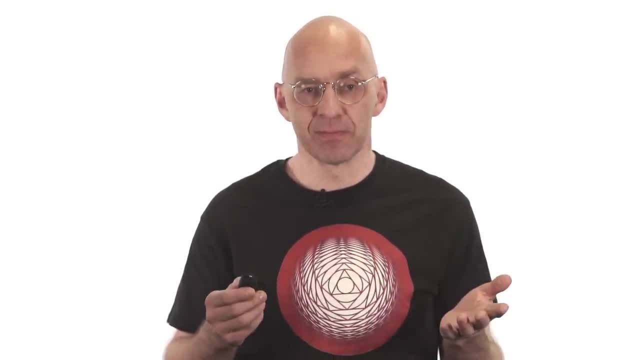 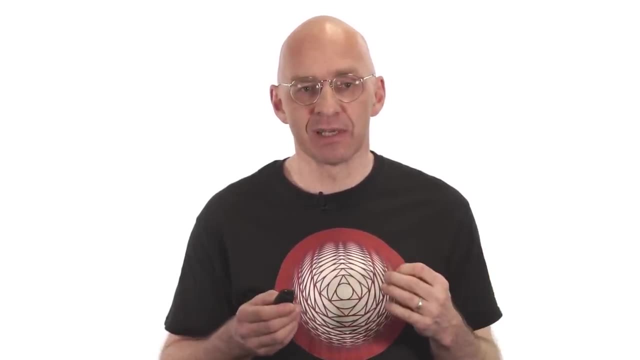 of the rules, such as the ones I have given in the video. Just like those people who write to me, there have been many thousands of people who've made this mistake over the years, and whole books have been written about their pointless endeavors To make absolutely sure that. 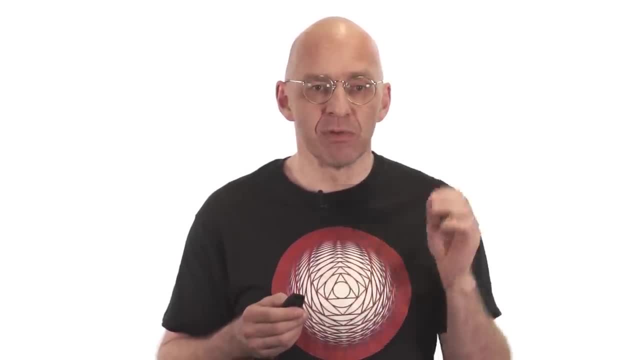 you really truly understand the rules and most definitely before you embark on the pointless quest of squaring the circle. I recommend you very carefully study those rules and the common mistakes people make interpreting them. The wiki page on ruler and compass constructions is a great subject. If you want to learn more about the rules of Euclid, please visit the link in the description.